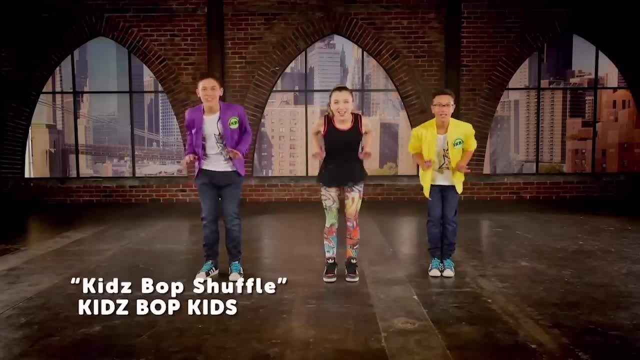 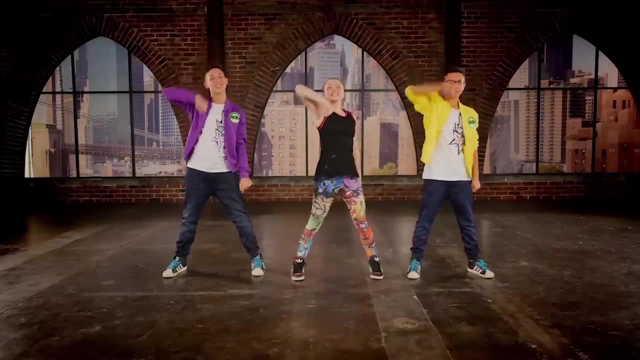 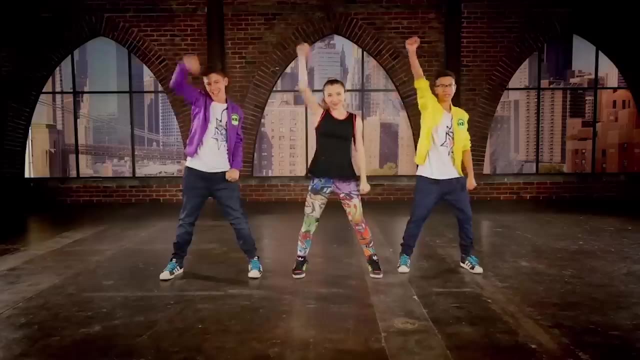 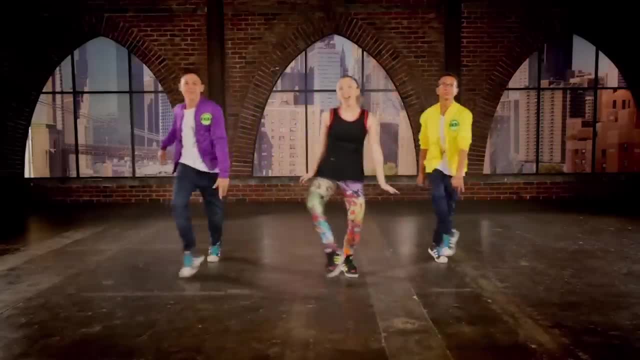 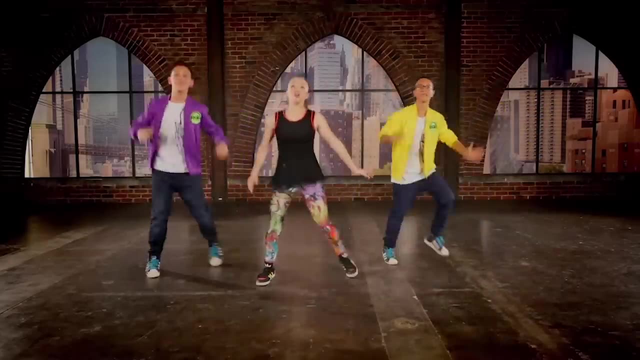 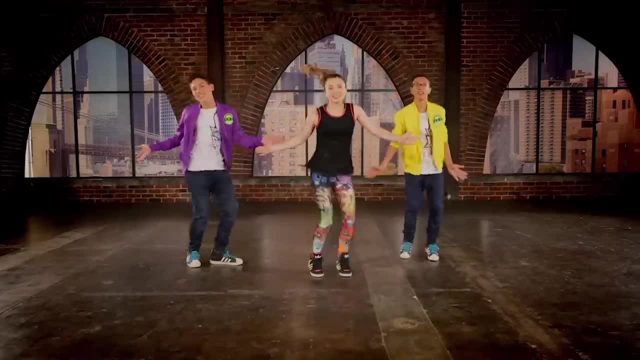 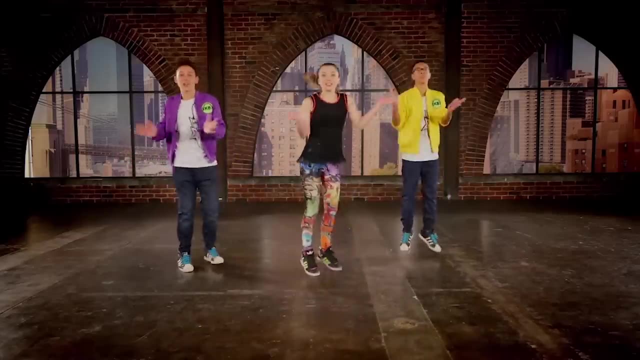 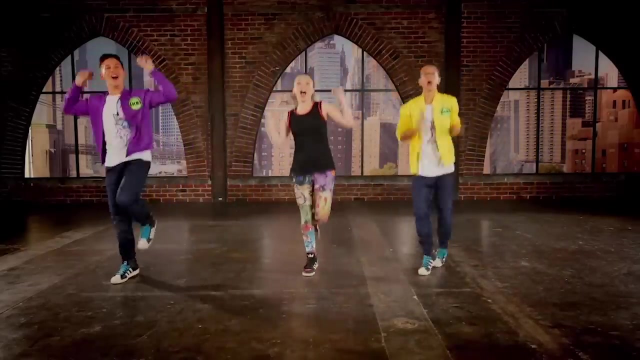 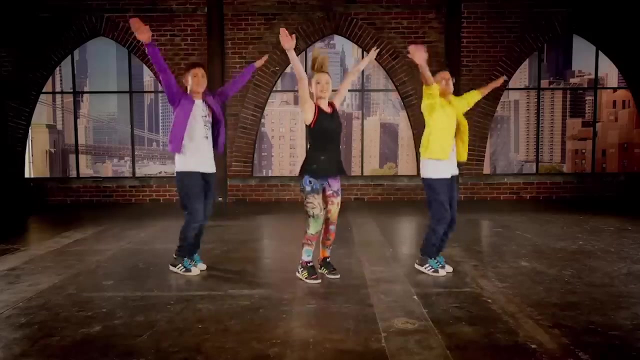 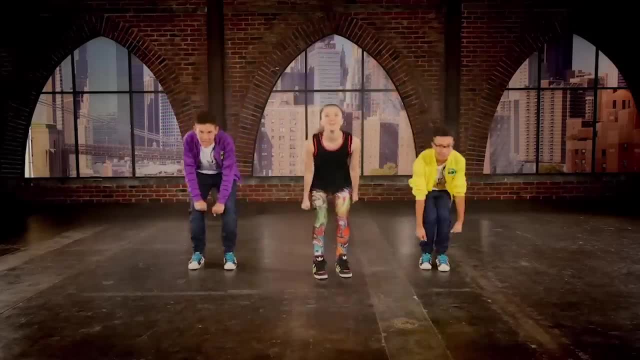 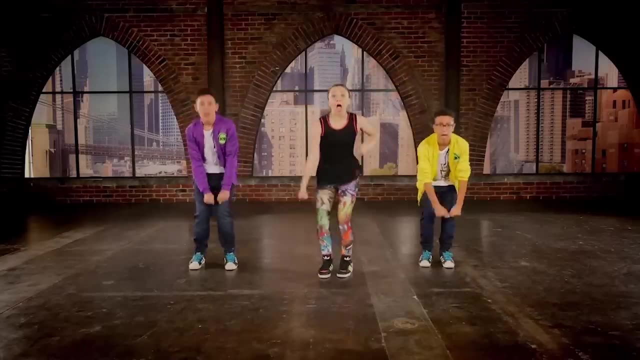 Moon M Allah Get on in, swing it back out. Kids rock the house. there is no doubt We're gonna show you what we're talking about. Down down Gia, dance Gia. Feel the kids bop. Down down Gia, dance Gia. 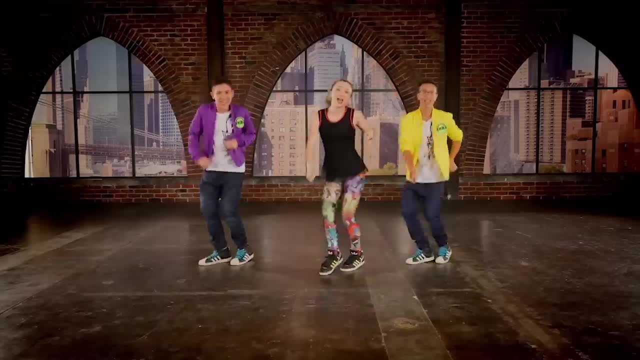 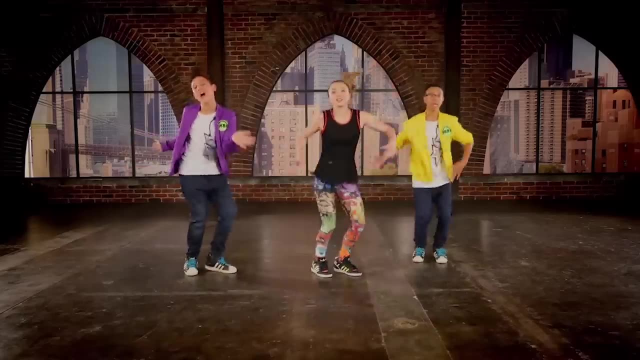 Let me see you do the Down down Gia, dance Gia. We got a brand new Down down Gia, dance Gia dance. Come on, Down down Gia, dance Gia. Feel the kids bop. 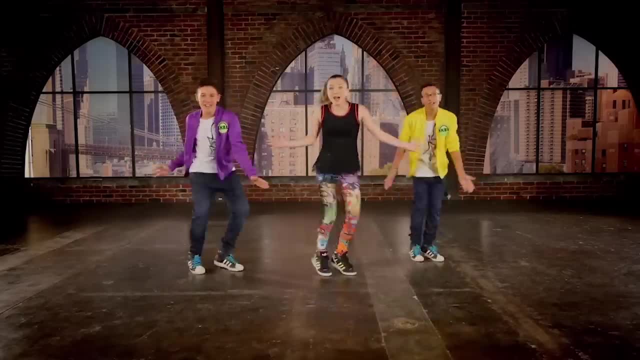 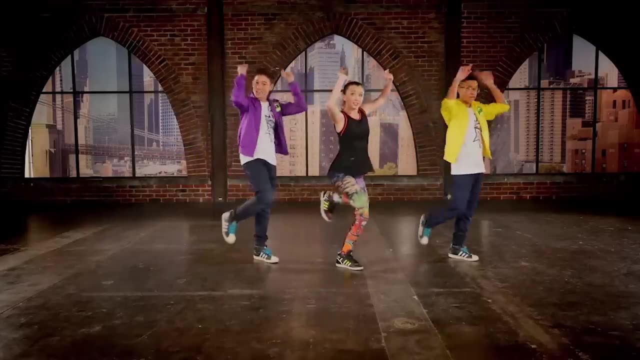 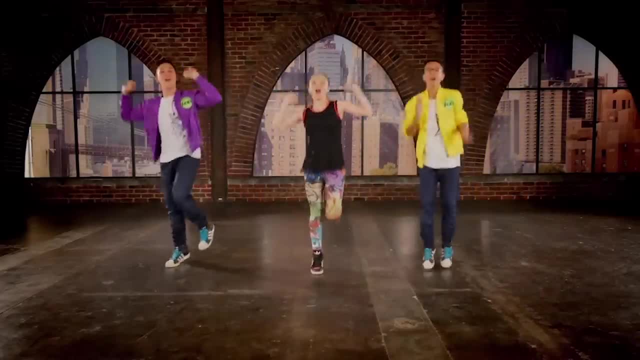 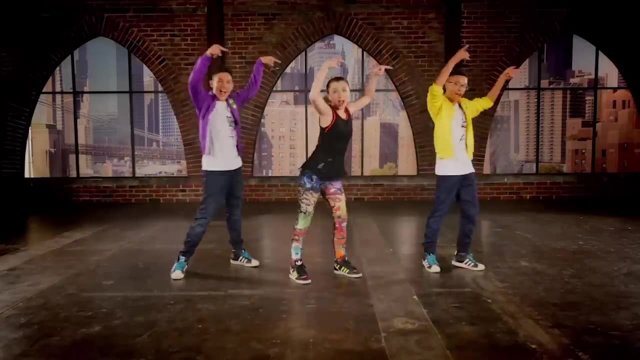 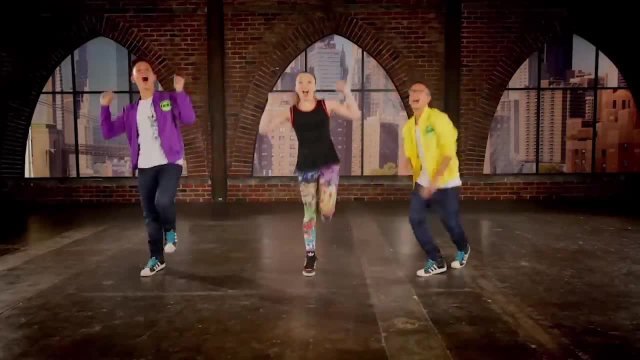 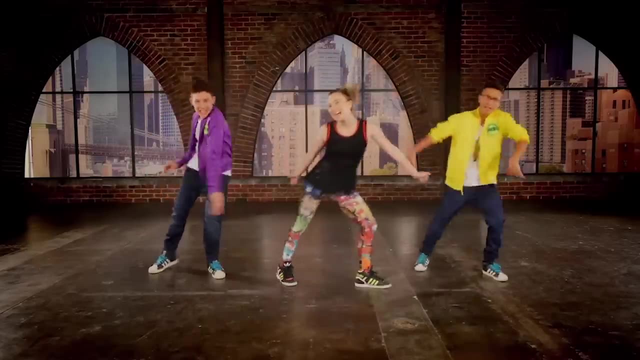 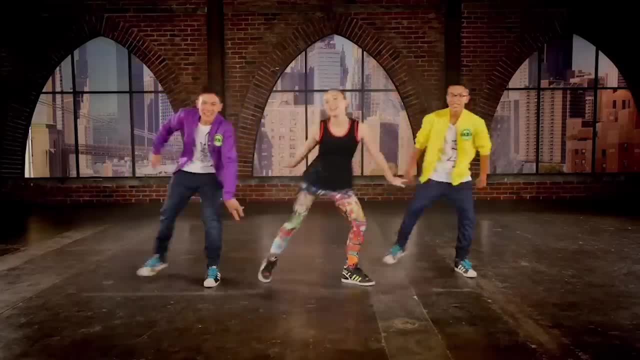 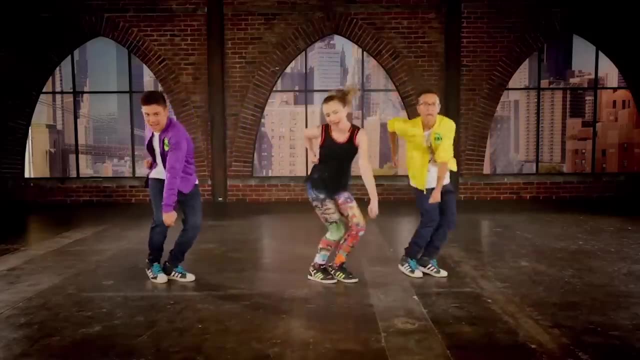 Kids bop shuffle. Now let me see you do the Kids from KBTTYLBRB. We're back on the track, got another Here we go. hey, Down down Gia, dance Gia. Feel the kids bop. Down down, Gia, dance Gia. 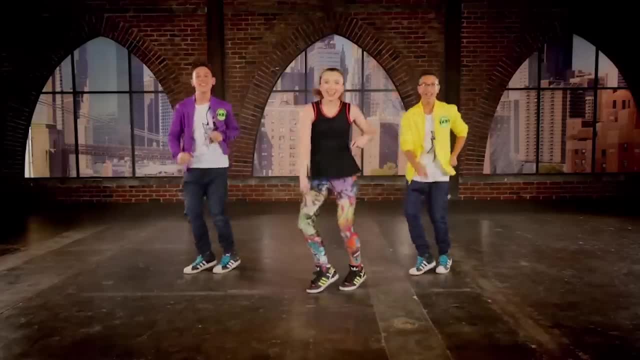 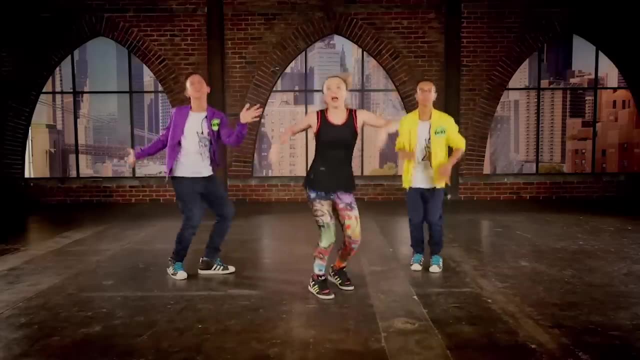 Let me see you do the Down down Gia, dance Gia. We got a brand new Down down Gia, dance Gia dance. Come on, Down down Gia, dance Gia. Feel the kids bop. 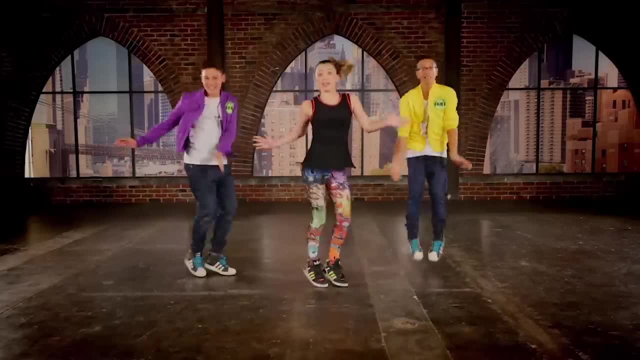 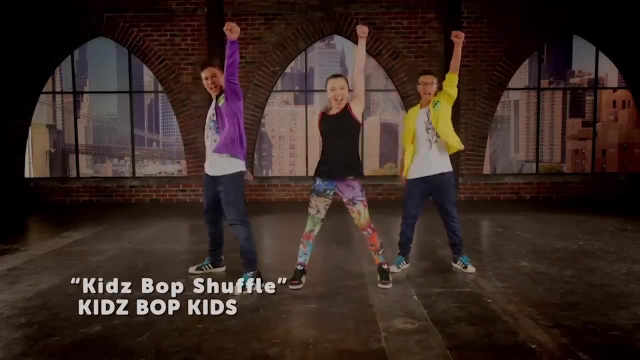 Down down Gia dance Gia. Let me see you do the Down down Gia dance Gia. We got a brand new Down down Gia dance Gia. We got a brand new style y'all. 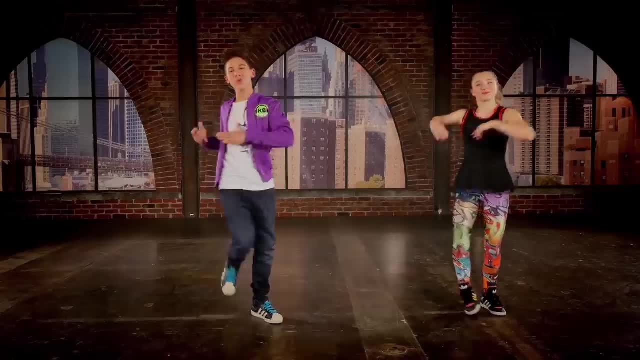 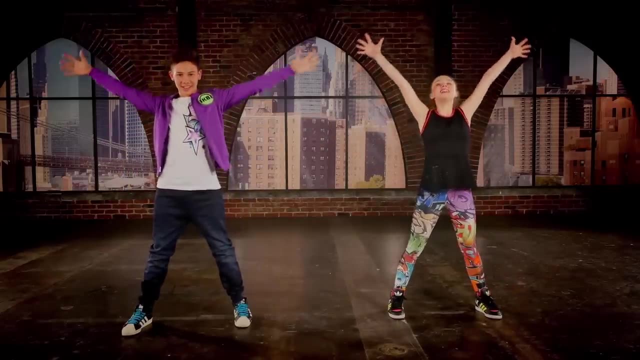 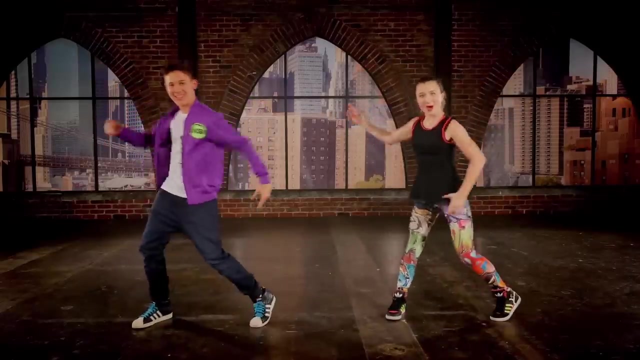 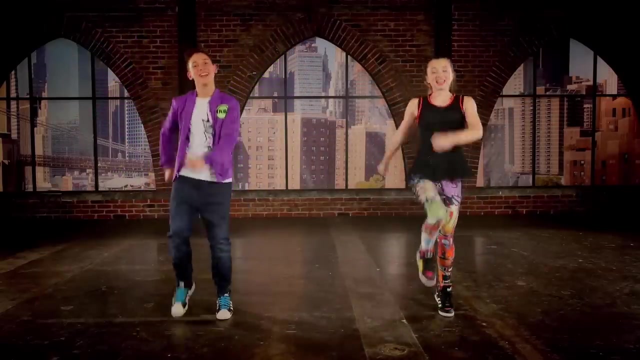 Like a small boat On the ocean Sending big waves Into motion, Like how a single wave Can make a heart open. I might only have one chance, But I can make an explosion. And all those things I didn't say Wrecking balls inside my brain. I will scream them loud tonight. 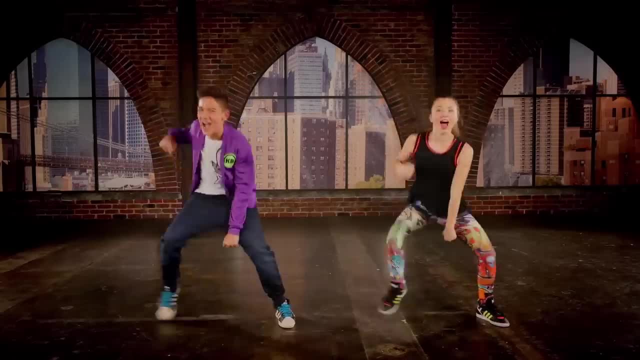 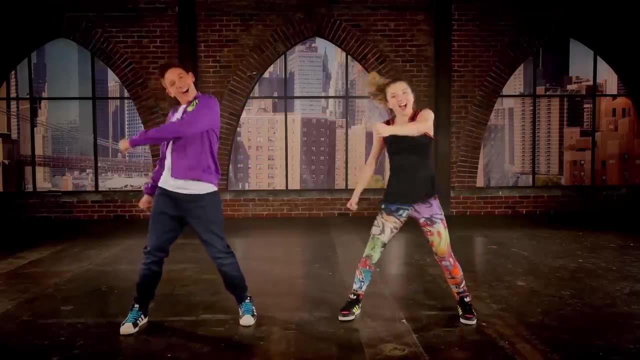 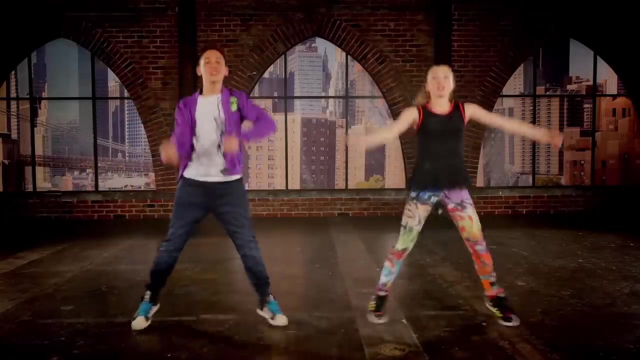 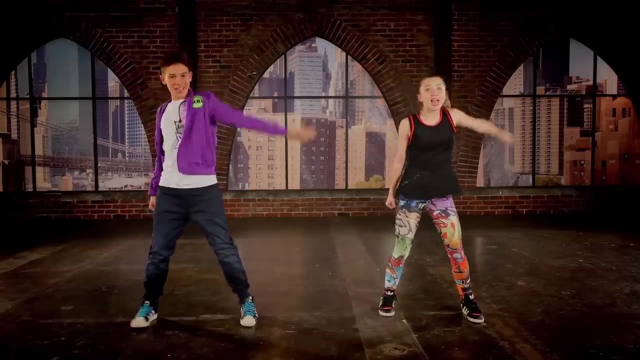 Can you hear my voice this time? This is my fight song. Take back my life So I can prove I'm alright. So My power's turned on. Starting right now, I'll be strong, I'll play my fight song And I don't really care What nobody else believes. 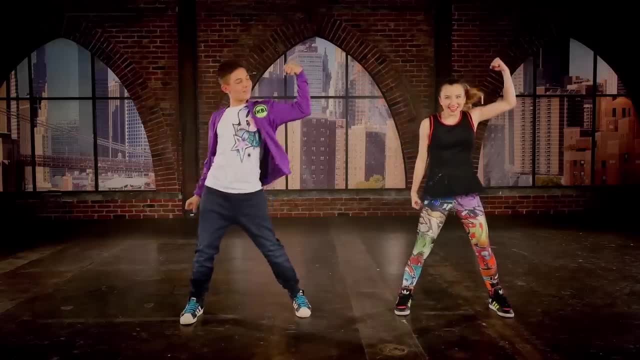 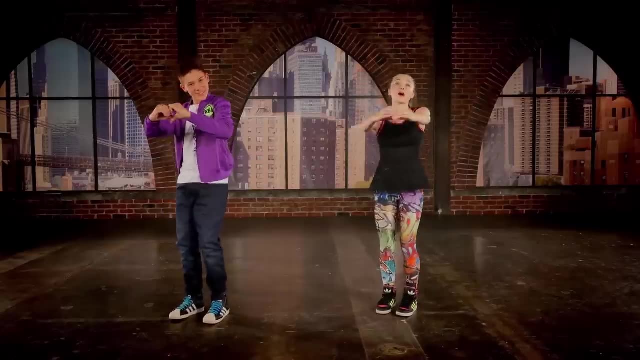 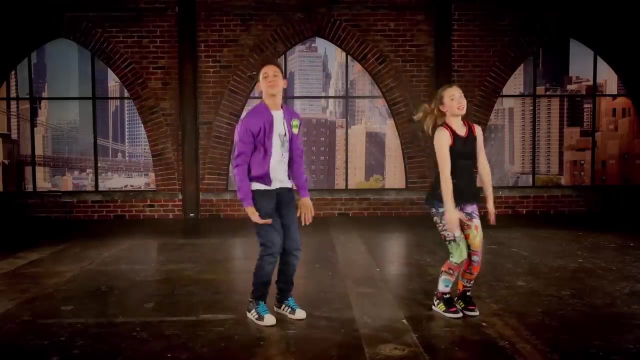 Cause I've still got A lot of fight left in me, Losing friends, And I'm chasing sleep. Everybody's worried about me In too deep, Say I'm in too deep, And it's been two years. I miss my home. There's a fire burning In my bones. And I still believe. Yeah, I still believe. And all those things I didn't say, Wrecking balls inside my brain. I will scream them loud tonight. Can you hear my voice this time? This is my fight song. Take back my life So I can prove. I'm alright. 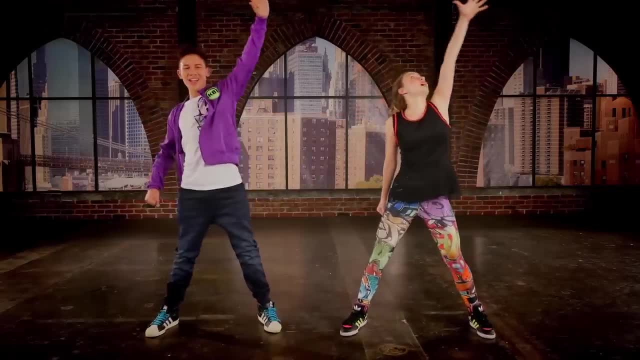 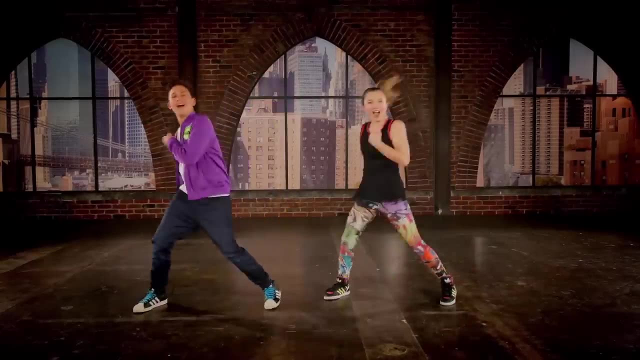 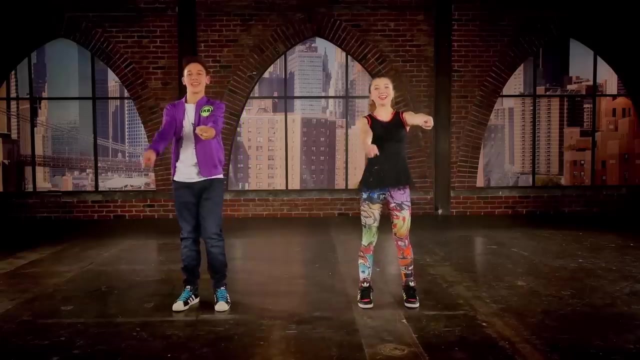 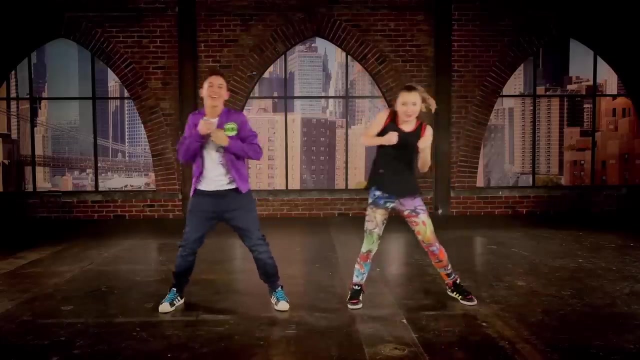 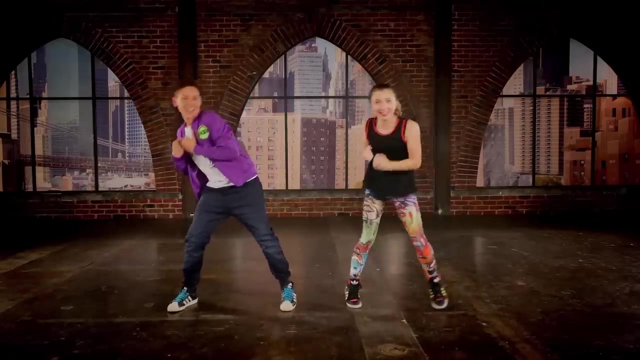 So My power's turned on. Starting right now, I'll be strong, I'll play my fight song, And I don't really care What nobody else believes, Cause I've still got A lot of fight left in me. A lot of fight left in me, Like a small boat. 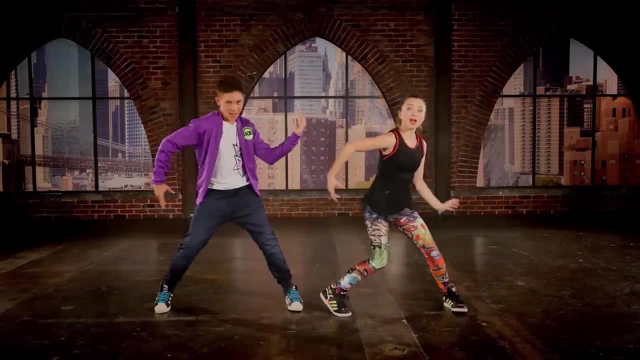 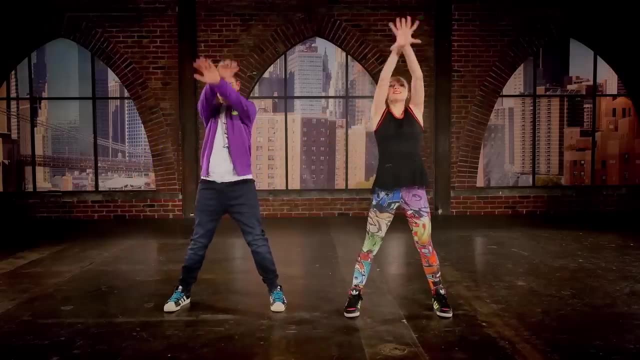 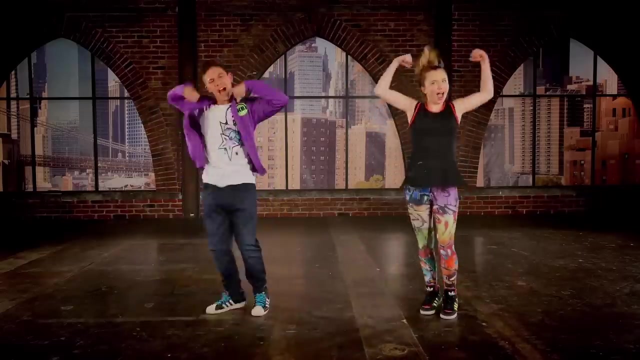 On the ocean. I might only have one chance, But I can make an explosion. This is my fight song: Take back my life And I still believe, Yeah, I still believe. And all those things I didn't say Wrecking balls inside my brain. I miss my home. 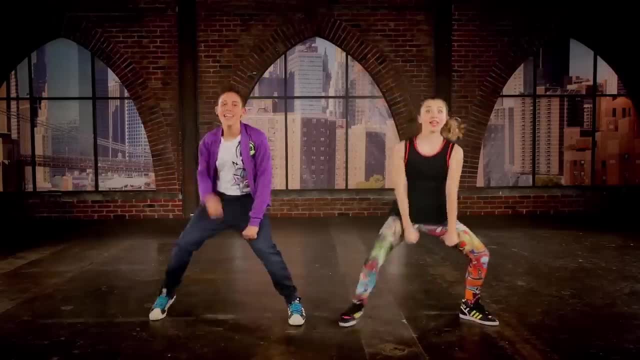 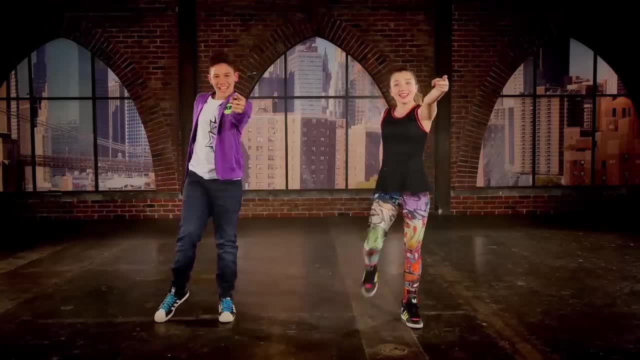 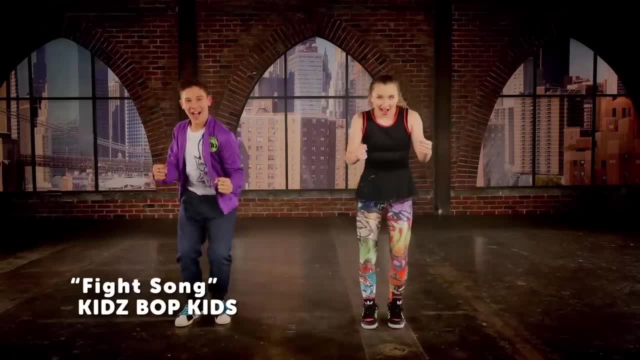 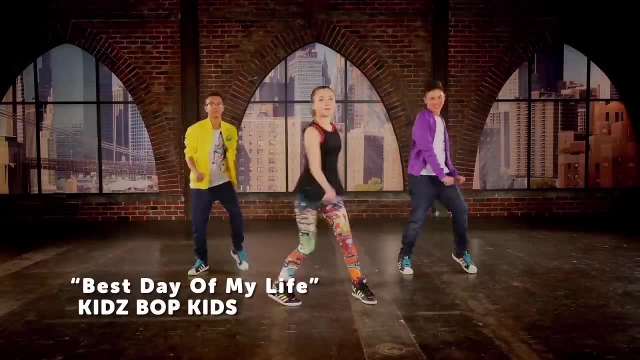 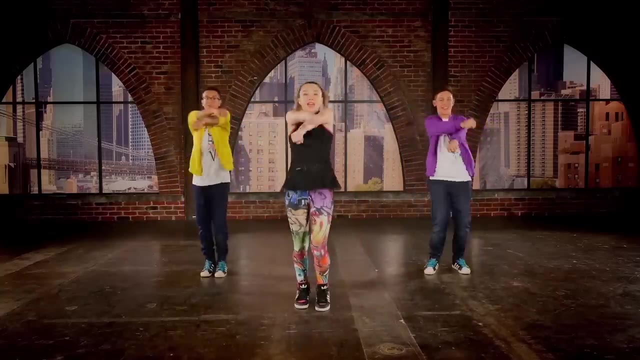 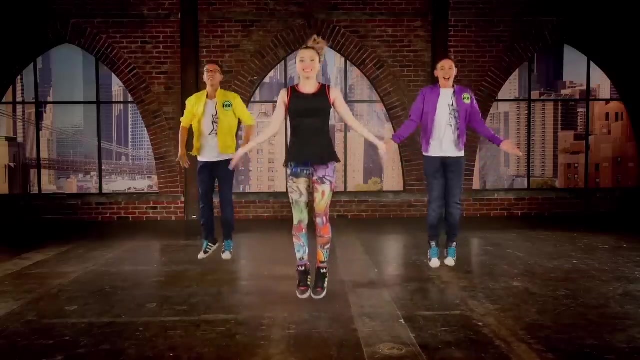 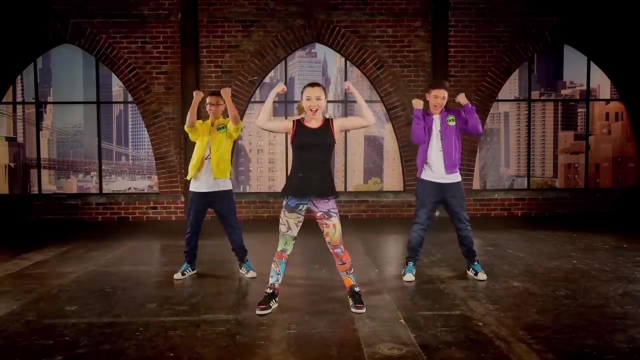 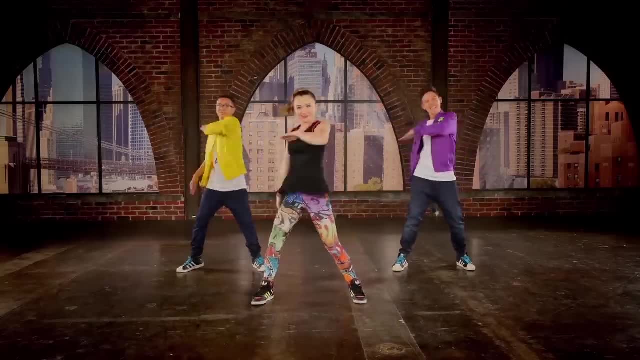 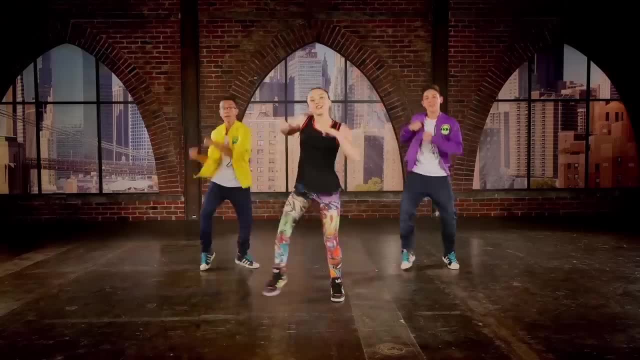 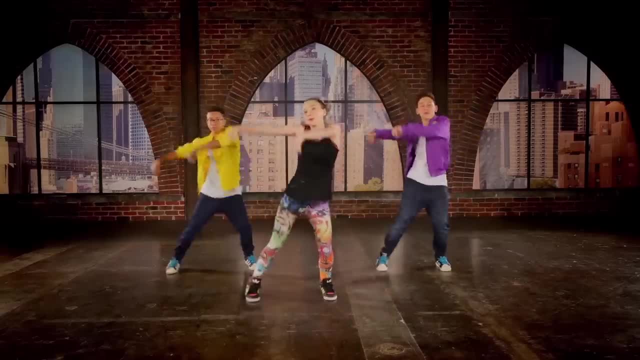 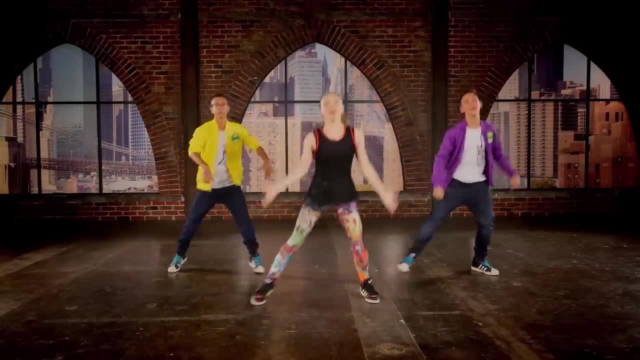 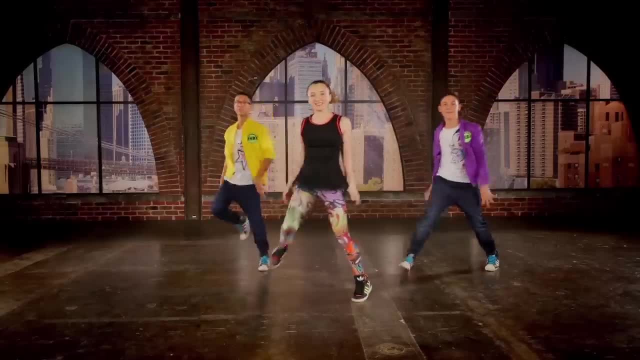 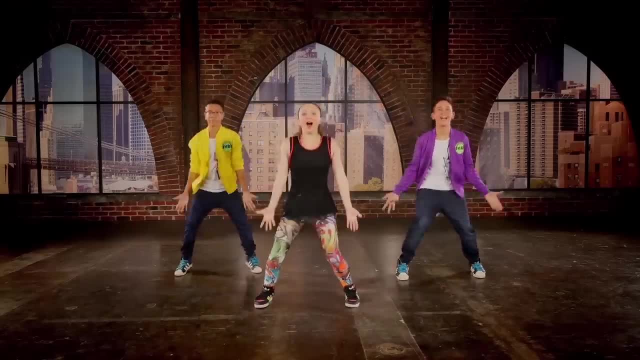 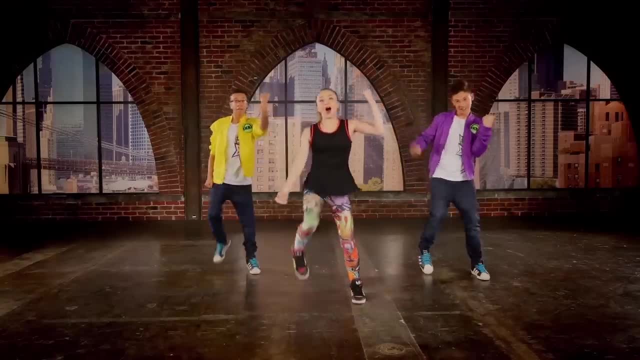 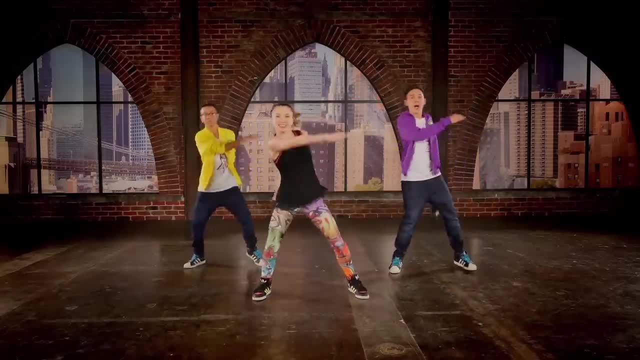 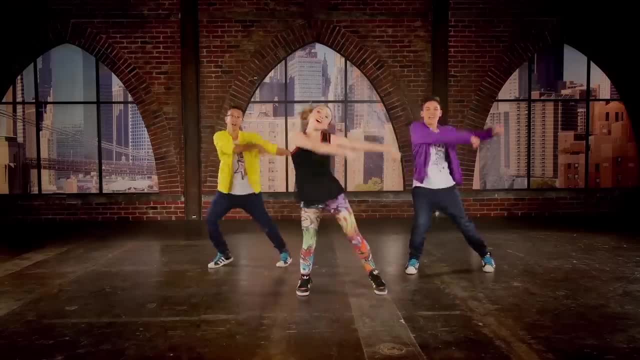 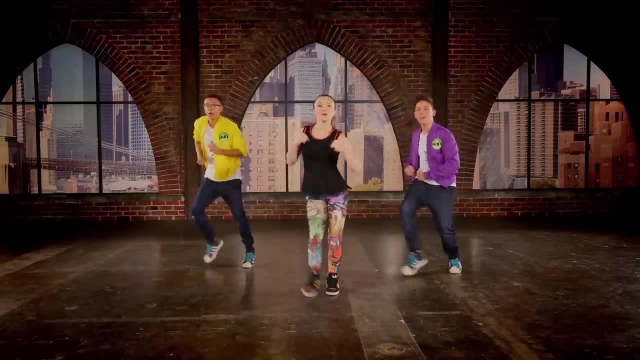 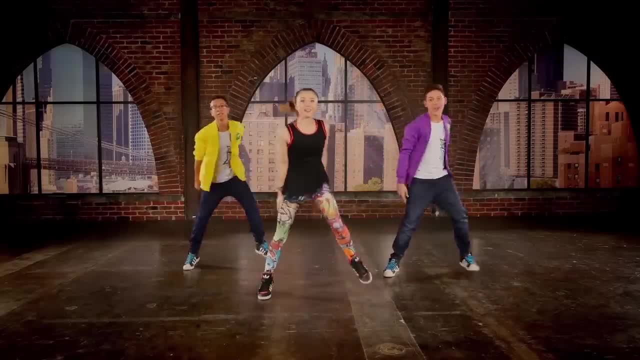 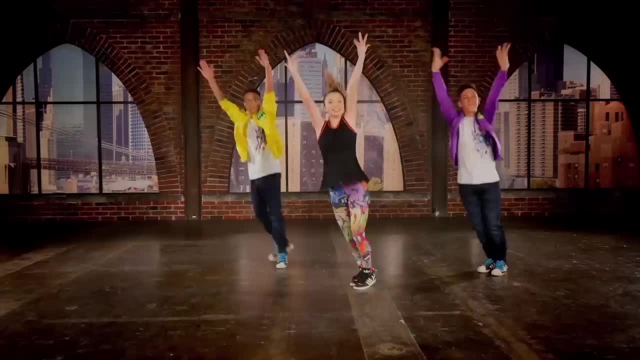 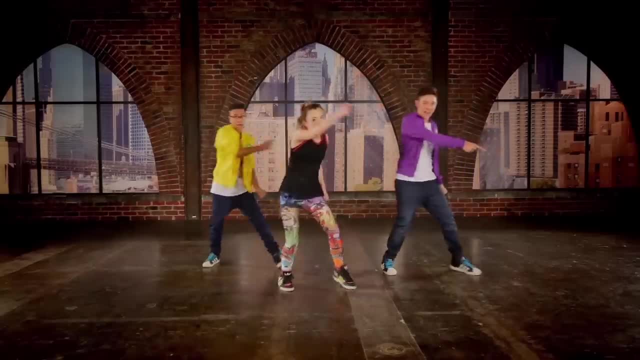 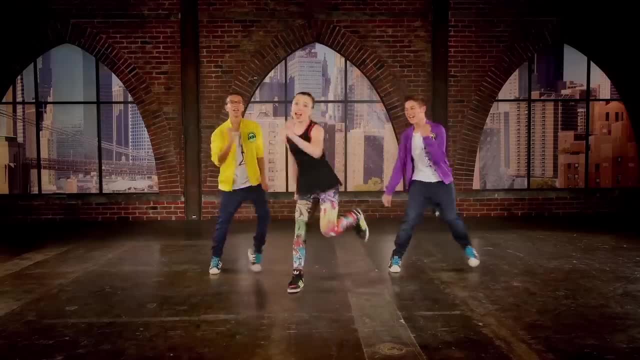 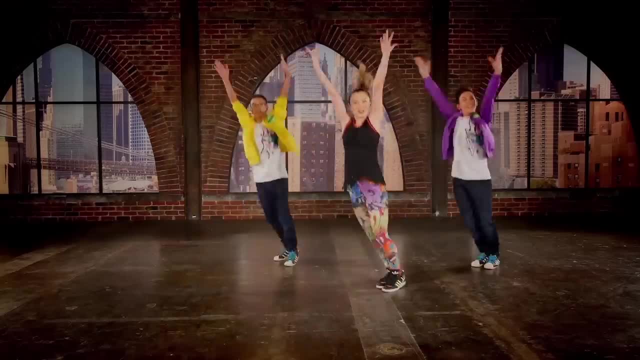 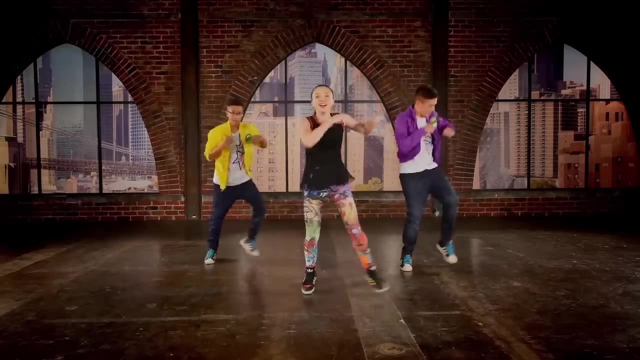 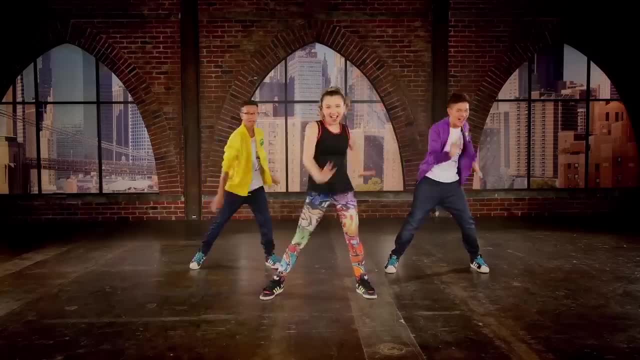 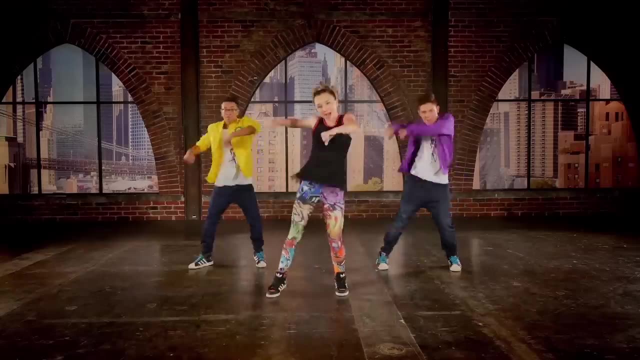 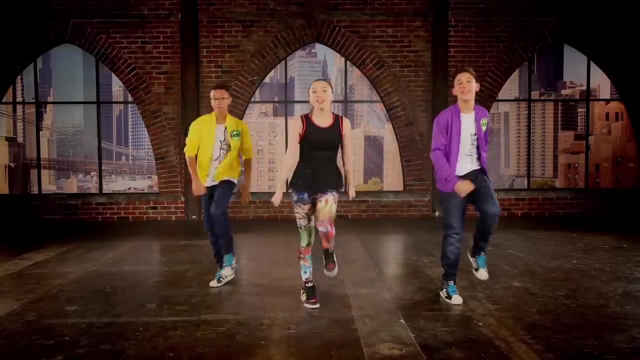 This is gonna be the best day of my life. My li-i-i-i-i-ife- Ooh, ooh, ooh, ooh. This is gonna be the best day of my life. My li-i-i-i-i-ife- Ooh, ooh, ooh, ooh. This is gonna be, this is gonna be, this is gonna be. 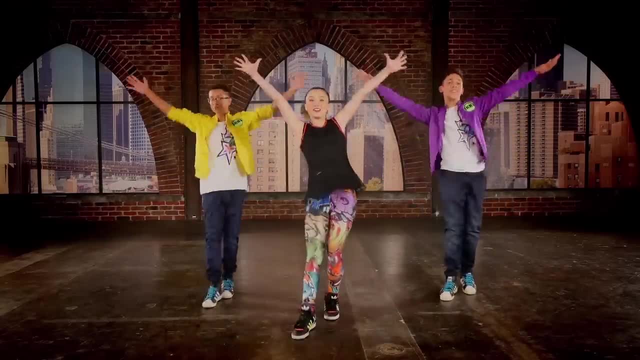 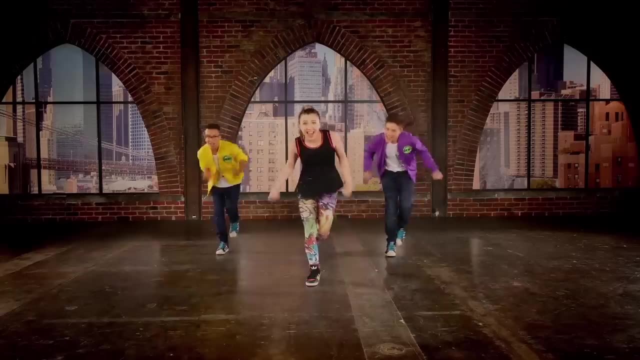 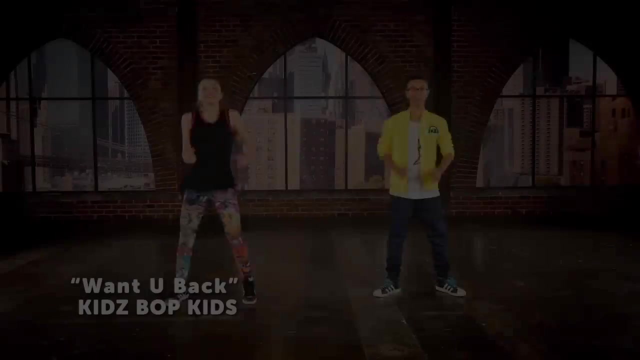 The best day of my life. Everything is looking up, everybody up now. Ooh, ooh, ooh, ooh. This is gonna be the best day of my life. My li-i-i-i-i-ife, Uh, Mm, yeah, La-la-la-la-la. 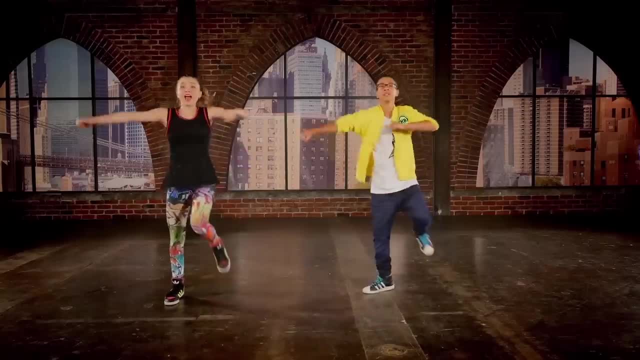 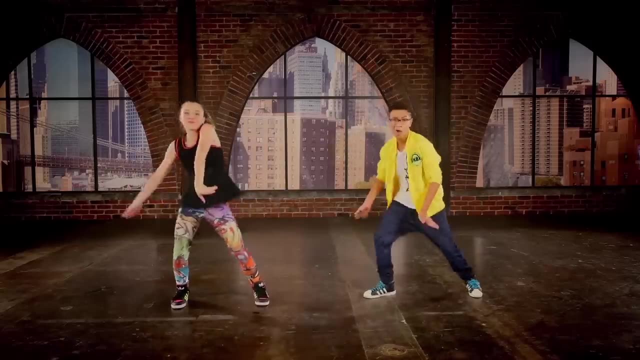 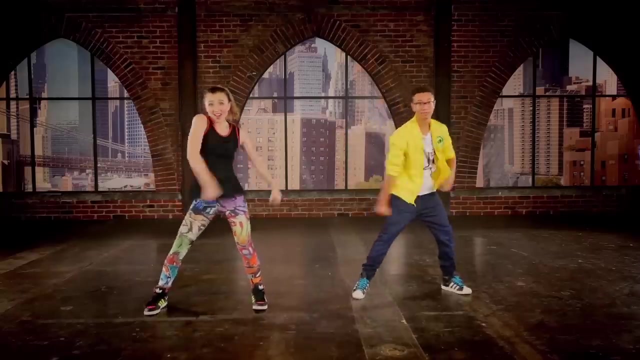 Ha-ha, Uh, Hey boy, you never had much game Thought I needed to upgrade, So I went and walked away way, way. Uh. Now I see you've been hanging out With that other girl in town Looking like a pair of clowns, clowns, clowns. 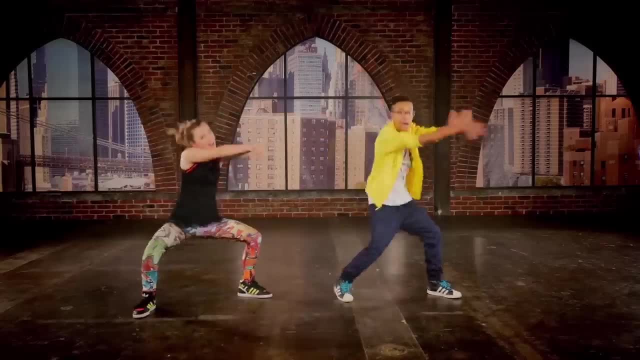 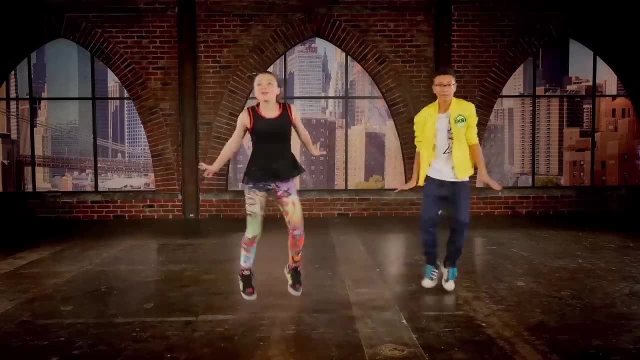 Uh, Remember all the things that you and I did first, And now you're doing them with her. Remember all the things that you and I did first. You got me, got me like this, Uh. And now you're taking her to every restaurant And everywhere we went. come on, And now you're taking her to every restaurant. You got me, got me like this: Uh, Boy, you can say anything you wanna, I don't care at all. no one else can have ya. I want you back. I want you back, Want, want you want you back. 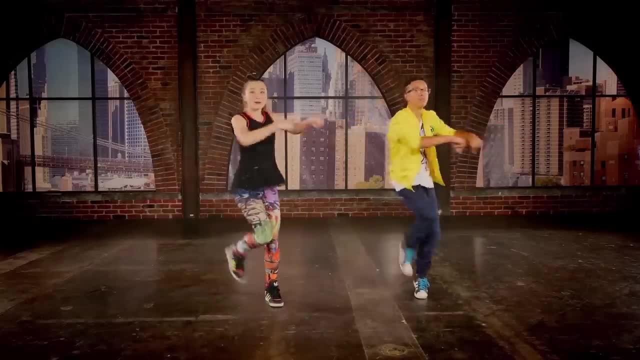 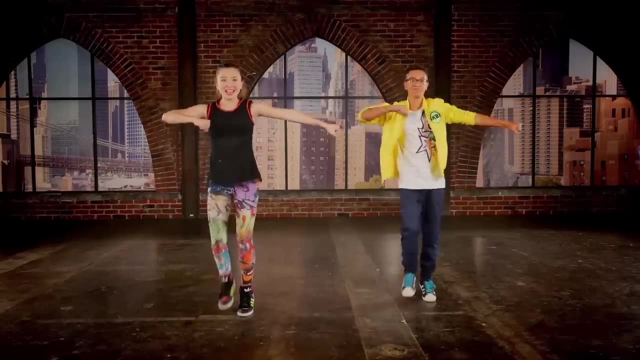 Uh, I broke it up thinking you'd be crying. Now I feel so bad looking at you flying. I want you back. I want you back, Want, want you, want you back. Uh, Please, this ain't even jealousy, Jealousy. She ain't got a thing on me. 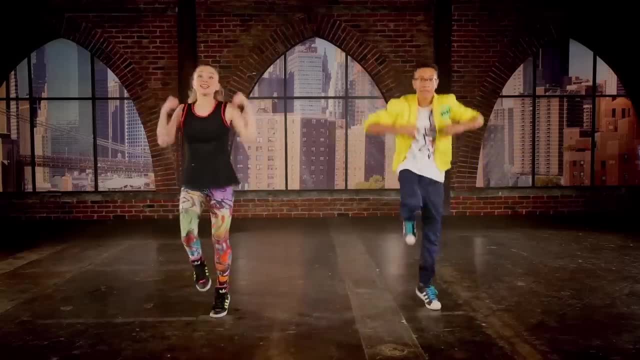 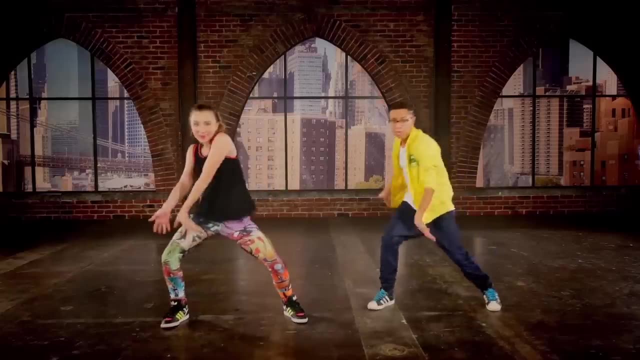 I ain't got a thing on me Trying to rock them ugly: jeans, jeans, jeans. Uh, You clearly didn't think this through. Yeah, what I've been told is true, Is it true? You'll be crawling back like boo. hoo, hoo, Uh. 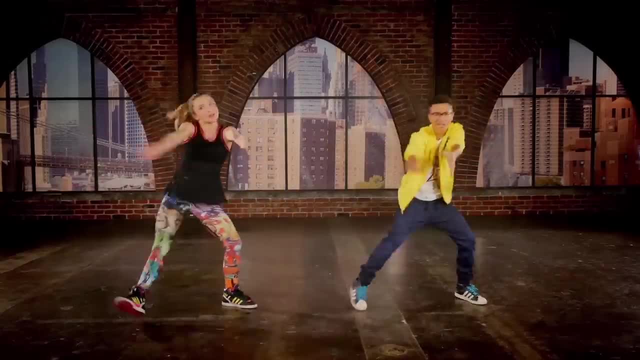 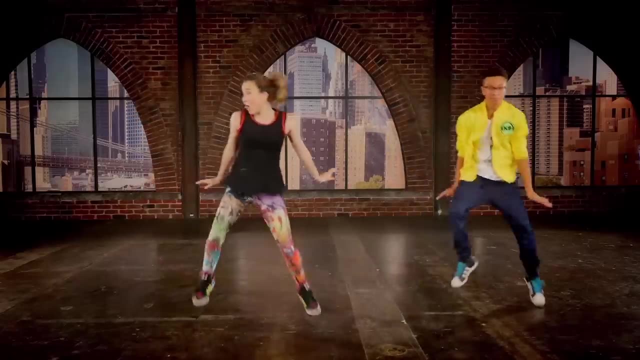 Remember all the things that you and I did first, And now you're doing them with her. Remember all the things that you and I did first. You got me, got me like this, Like this, Uh. And now you're taking her to every restaurant, Yeah, And everywhere we went. come on. 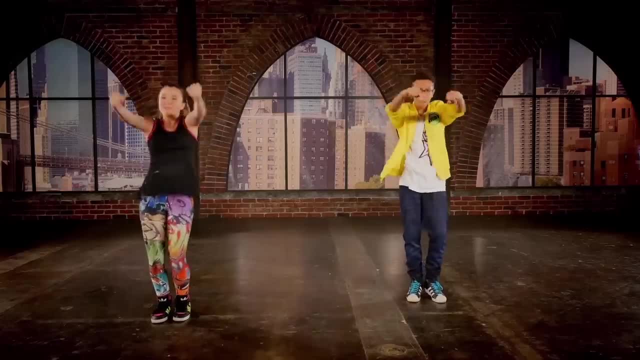 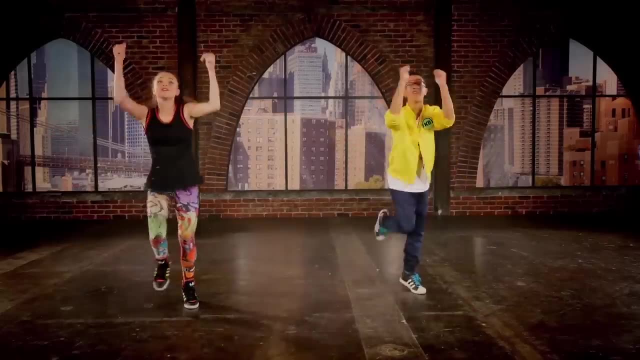 And now you're taking her to every restaurant. You got me, got me like this: Uh, Boy, you can say anything you wanna, I don't care at all. no one else can have ya. I want you back. I want you back, Want, want you want you back. 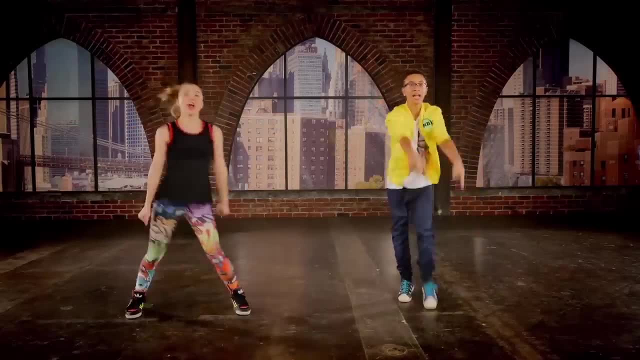 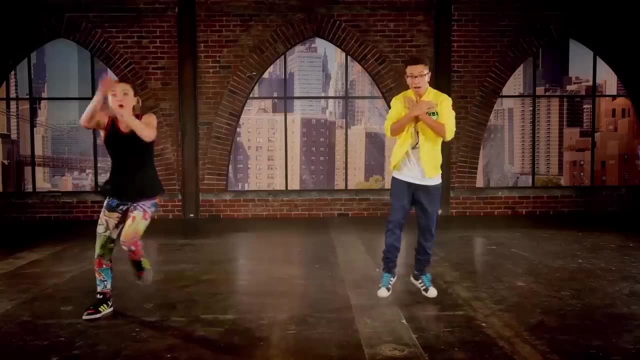 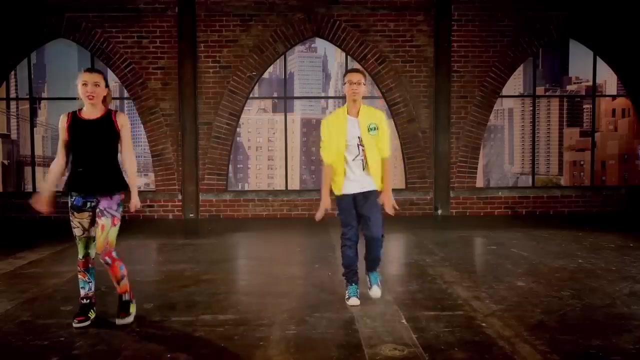 Uh, I broke it up, thinking you'd be crying. Now I feel so bad looking at you flying. I want you back. I want you back, Want, want you. want you back. Uh, Ooh, I thought you'd still be mine When I kissed you goodbye. 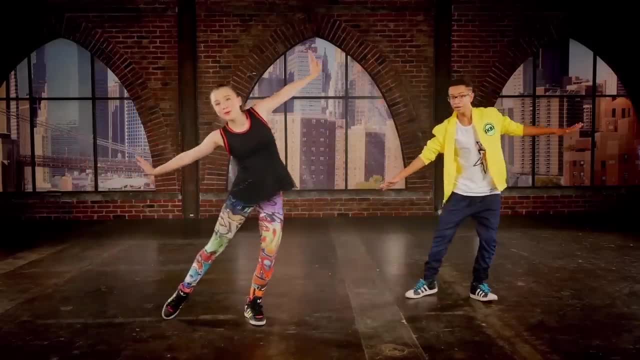 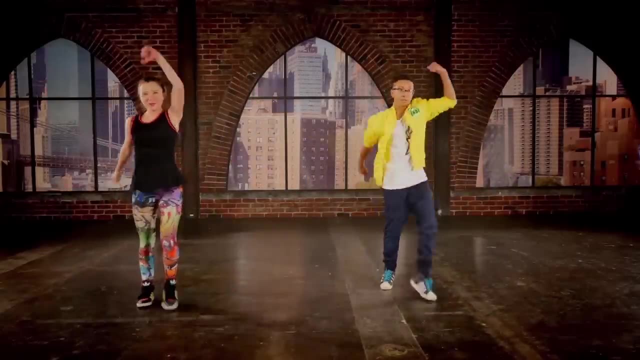 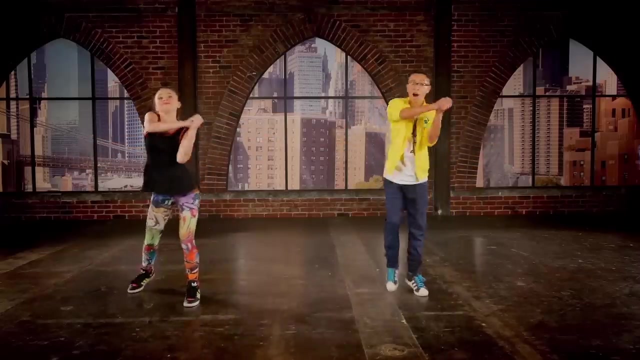 Oh, oh, oh, oh, Ooh, And you might be with her, But I still had you first. Oh, oh, oh oh. Remember all the things that you and I did first, And now you're doing them with her. Remember all the things that you and I did first. 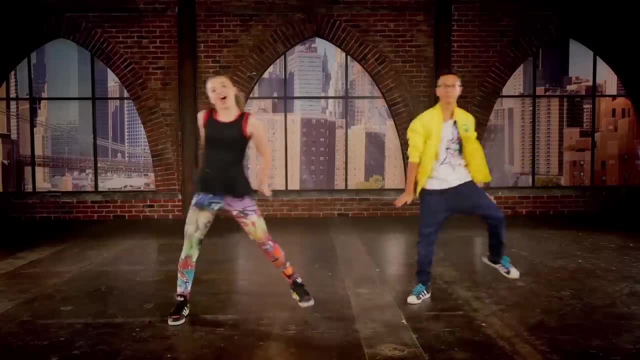 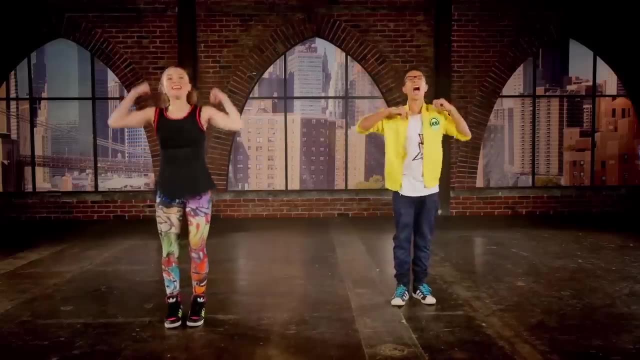 Yo, Remember all the things that you and I did first, And now you're doing them with her. Remember all the things that you and I did first. You got me, got me like this: Uh Boy, you can say anything you wanna, I don't care at all, no one else can have ya. 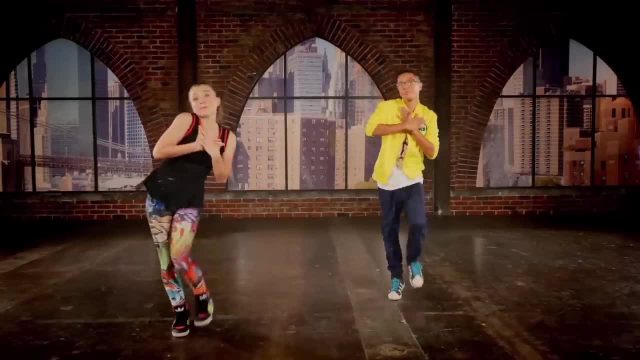 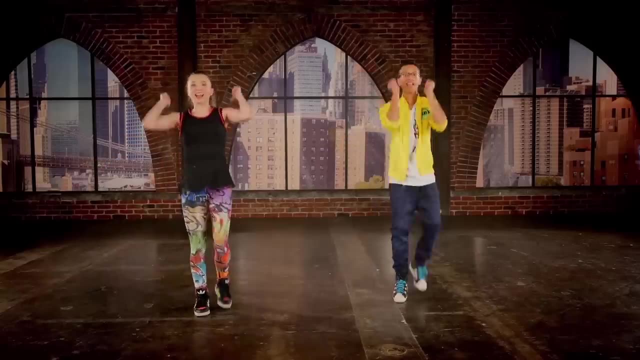 I want you back. I want you back, Want, want you, want you back. Uh, I broke it up thinking you'd be crying Now I feel so bad looking at you flying. I want you back. I want you back, Want, want you. want you back. 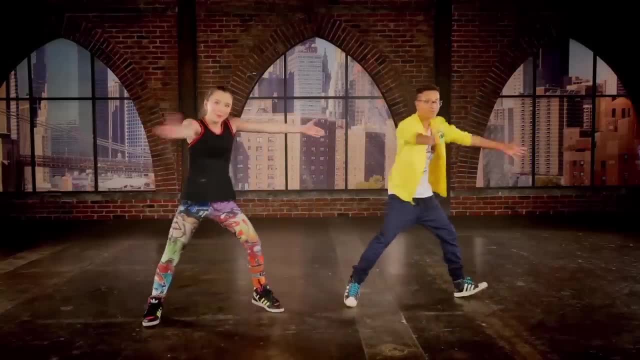 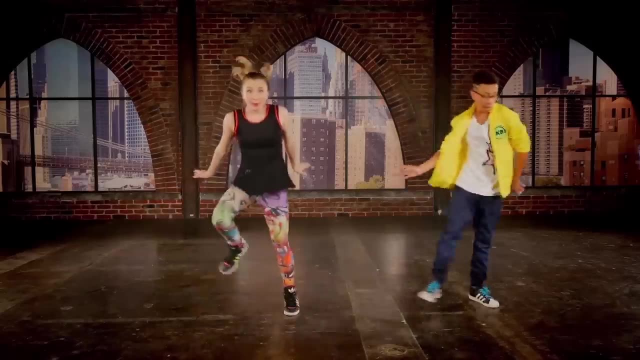 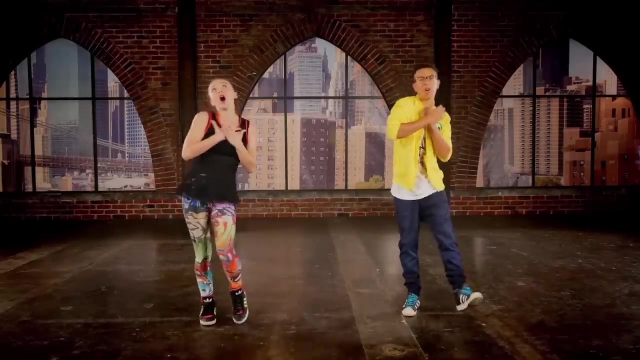 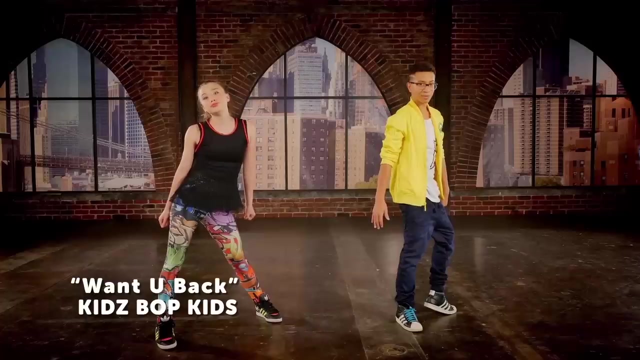 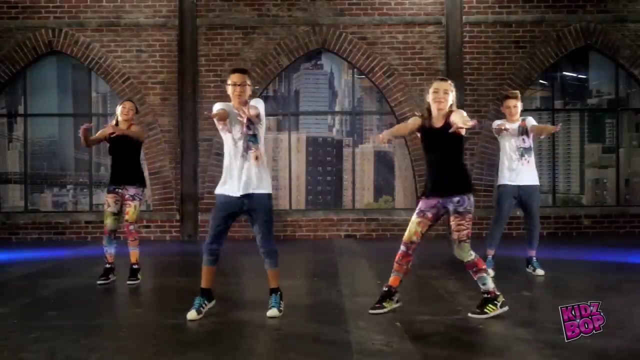 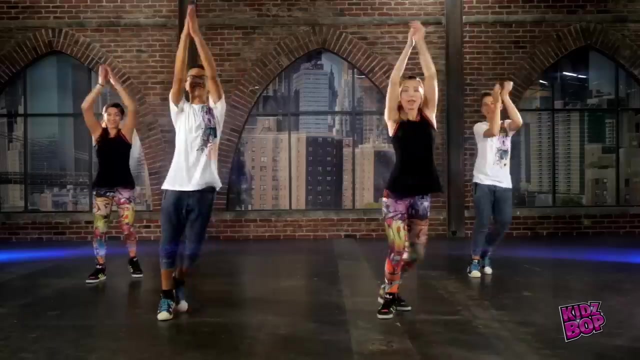 I want you back. I want you back. I want you back. Want, want you, want you back. Uh, Ooh, I want you back. I want you back. Want, want you, want you back. Uh, Do I sound like a helicopter? Uh, Oh, sometimes I get a good feeling, yeah. 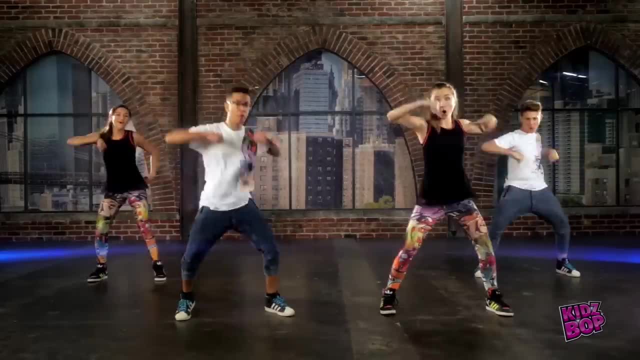 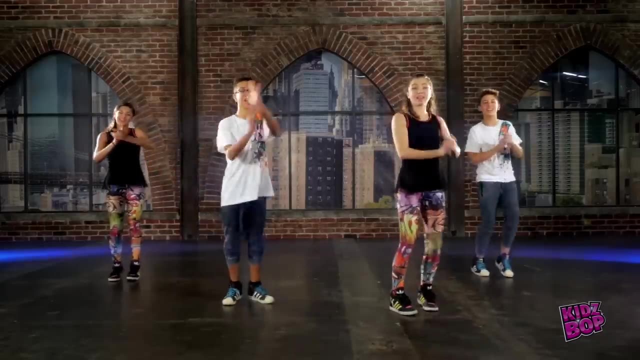 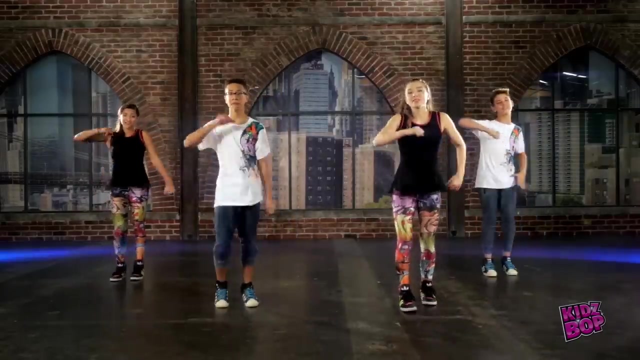 I get a feeling that I never, never, never, never had before. No, no, I get a good feeling, yeah. Oh, sometimes I get a good feeling. yeah, I get a feeling that I never, never, never, never had before. No, no, I get a good feeling, yeah. 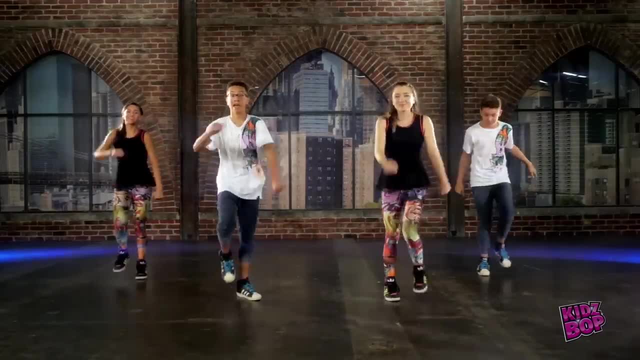 Yes, I can Doubt that I'll leave. I'm running with this plan. Pull me, grab me. crabs in a bucket can't have me. I'll be the president one day, January 1st. are you like that guy? I said 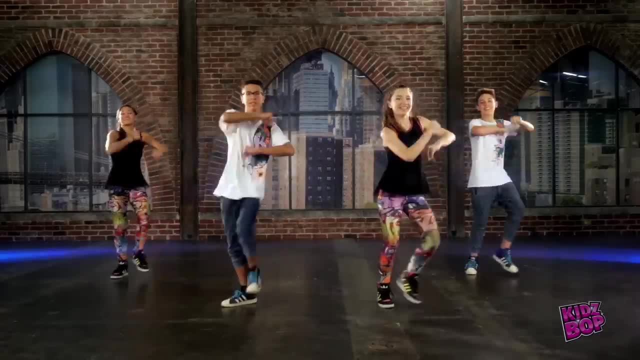 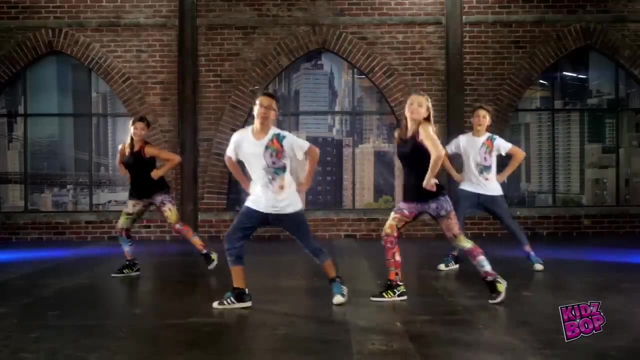 Are you the one thinking: what guy I said got done. Now I gotta work with the song. How many rolling stones you want? Yeah, I got a brand new spirit, vegan and stunned Woke up on the side of the bed like I won, Talked like a wind on my chest to that sun. 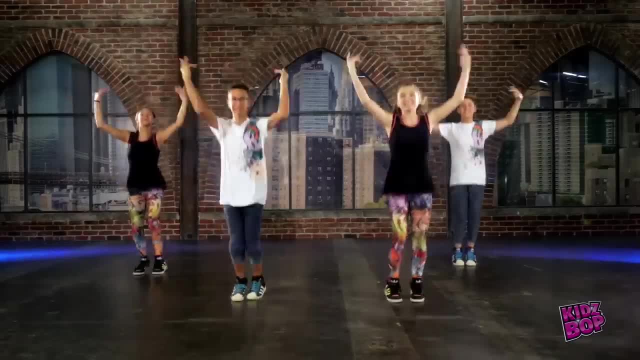 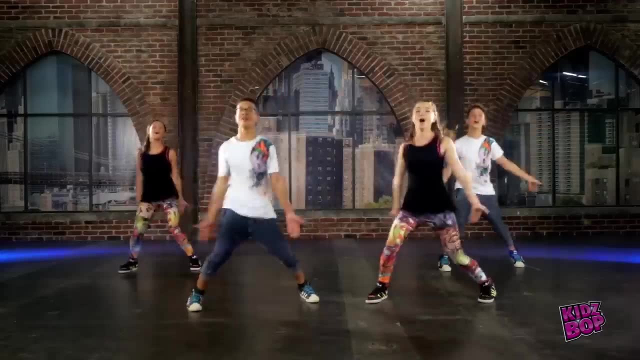 G5 dealer US to Taiwan. I hope you say that I wanna play it back. Mama knew I was a needle in a haystack. I'll be ready boy. plus payback. I got a feeling it's a wrap ASAP. Oh, sometimes I get a good feeling, yeah. 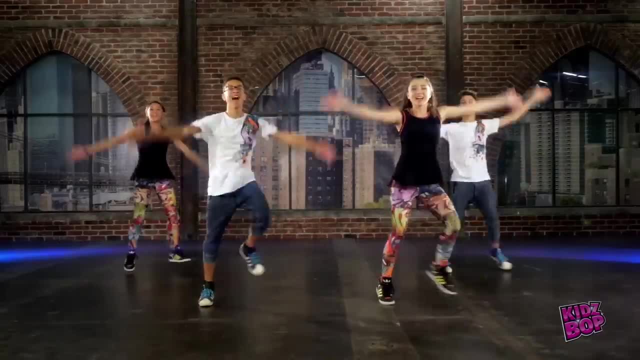 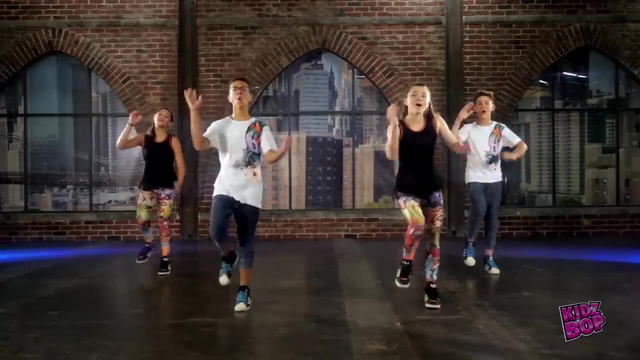 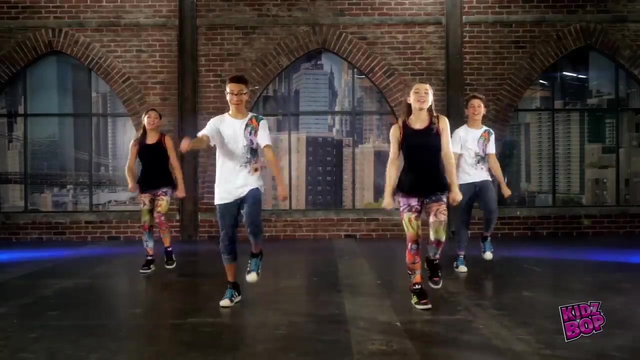 I get a feeling that I never, never, never, never had before. No, no, I get a good feeling, yeah, Oh, sometimes I get a good feeling. yeah, I get a feeling that I never, never, never, never had before. 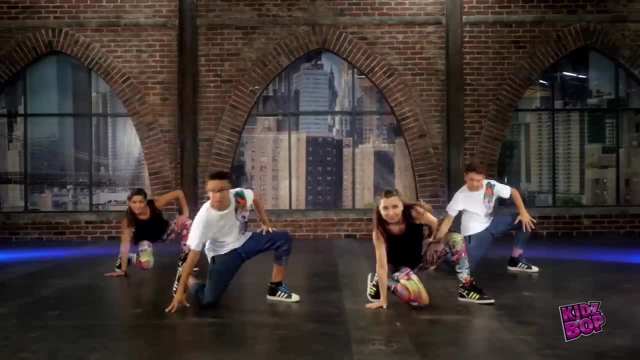 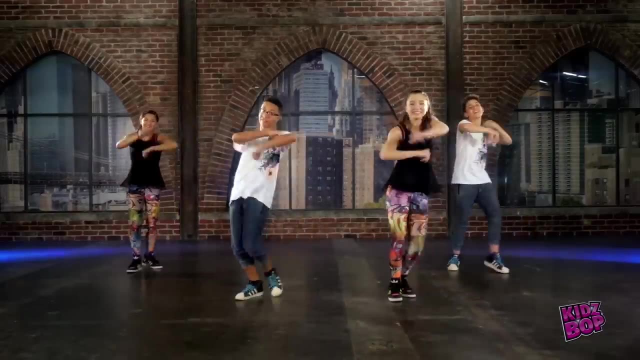 No, no, I get a good feeling. yeah, The mountaintop walk on water. I got power. feel so royal. One second I'ma strike oil Diamond platinum. no more for you. Gotta drill the land, never giving in. 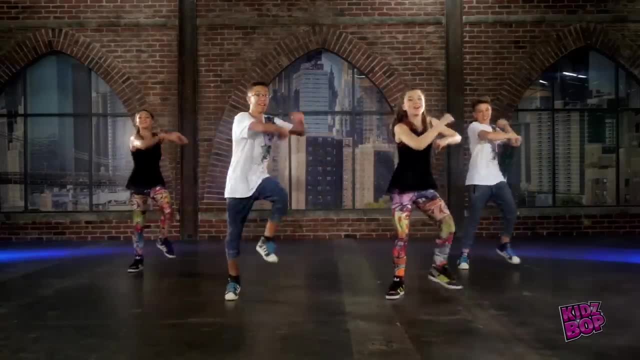 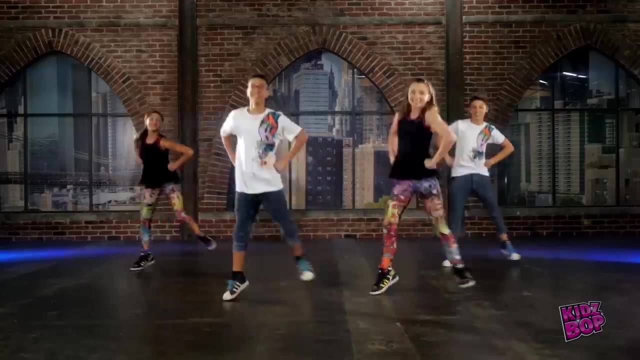 Giving up's not an option. gotta get it in Witness. I got the heart of 20 men. No fear gonna sleep in the lion's den. That soul that sparked that crown. You're looking at, the king of the jungle. now. I'm stronger than ever. can't hold me down. 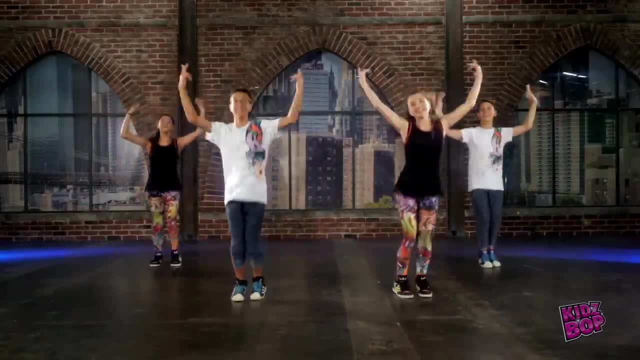 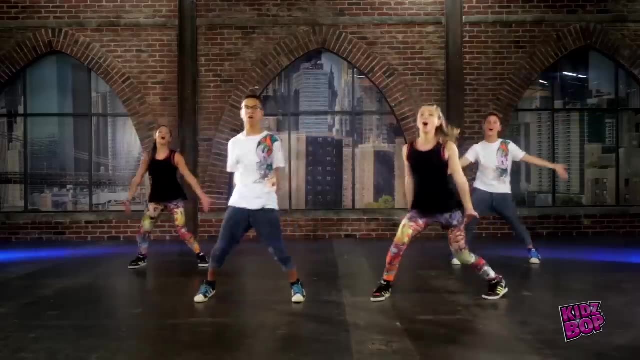 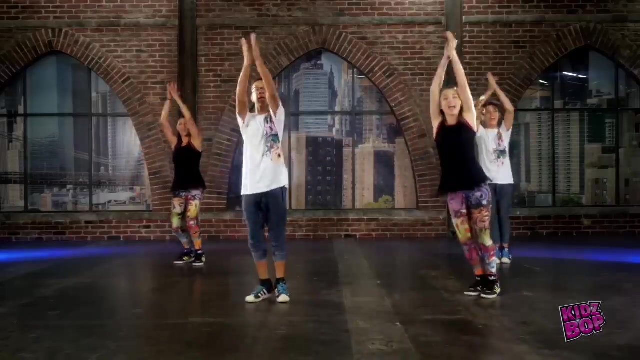 A hundred miles going from the picture. smile, Straight, game face. it's game day. See me run through the crowd full of melee. No trick plays. I'm Bill Gates. Take a genius to understand me. Oh, sometimes I get a good feeling. yeah, I get a feeling that I never, never, never, never had before. 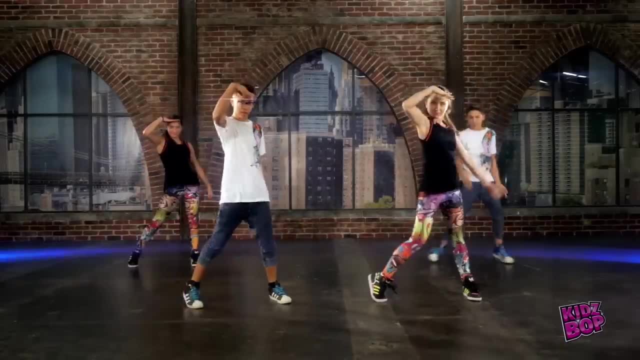 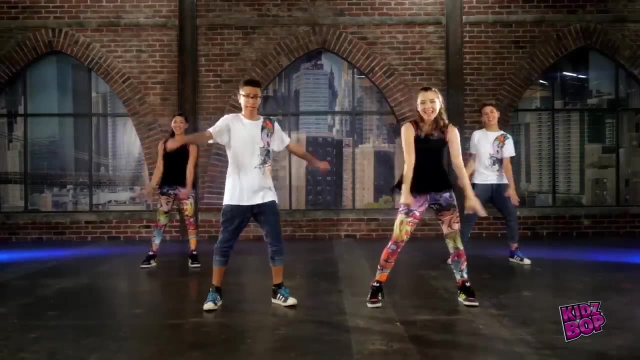 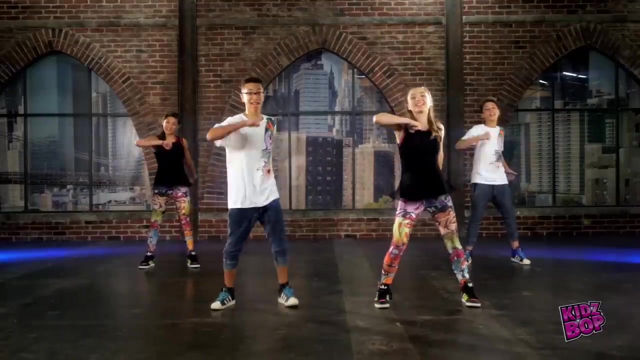 No, no, I get a good feeling. yeah, I know you got the good feeling. let's get it, let's get it. Gotta love the life that we livin'- let's get it, let's get it. I know you got the good feeling. let's get it, let's get it. 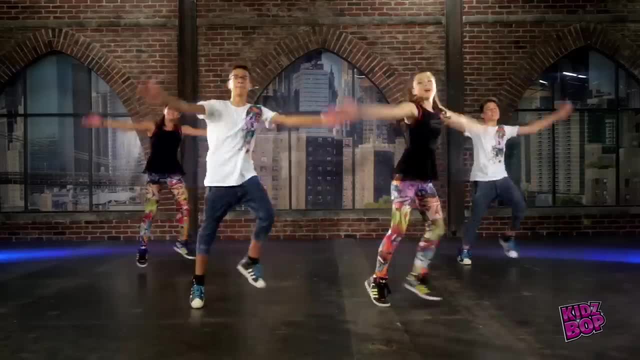 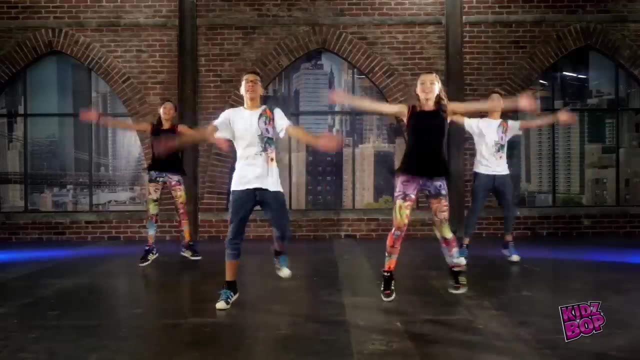 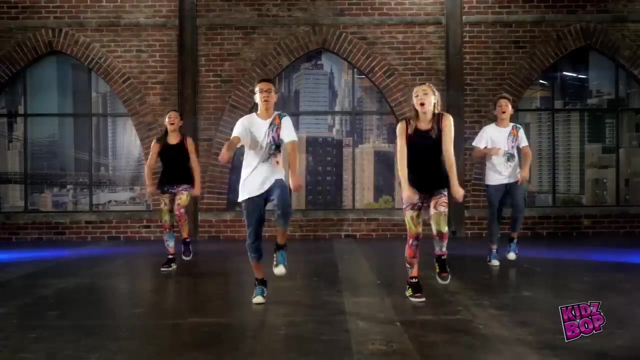 Gotta love the life that we livin'. oh, Sometimes I get a good feeling. yeah, I get a feeling that I never, never, never, never had before. No, no, I get a good feeling. yeah, Oh, sometimes I get a good feeling, yeah. 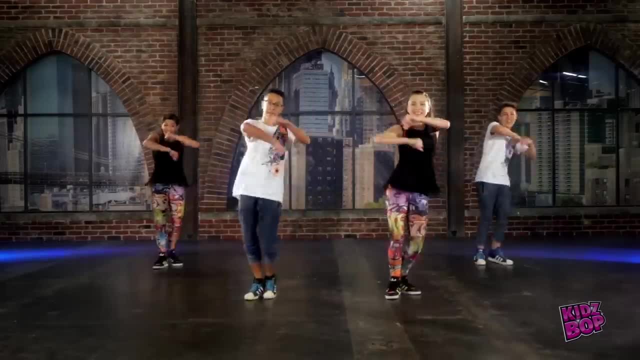 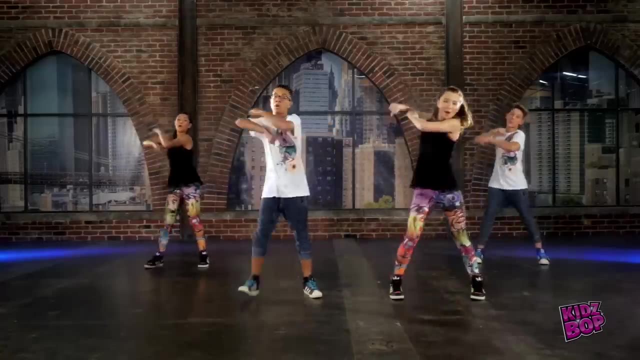 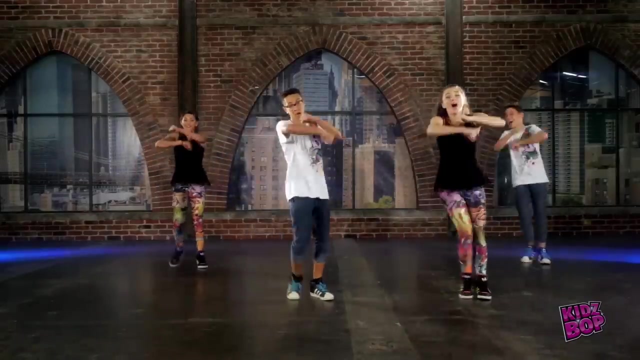 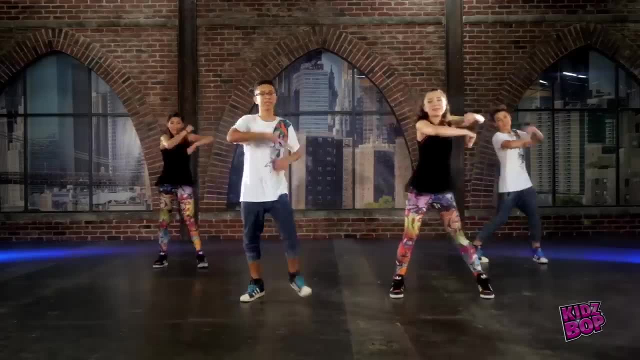 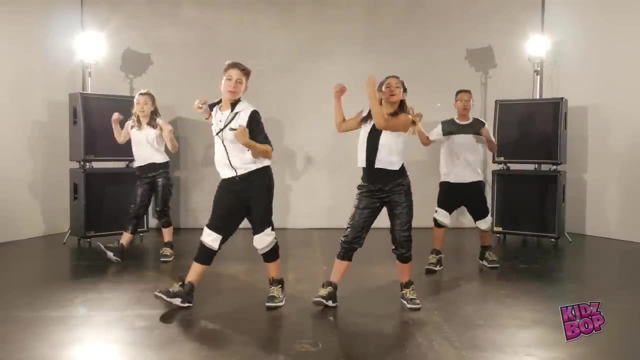 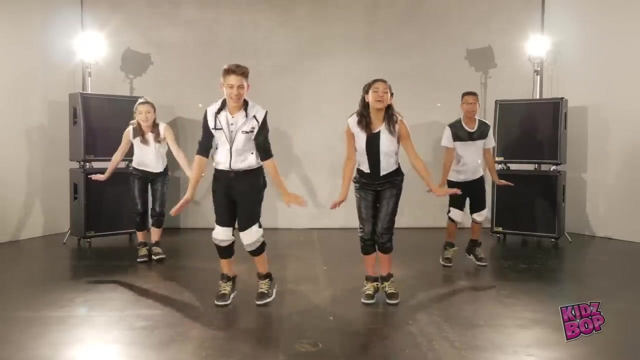 Oh, oh, oh oh. Sometimes I get a good feeling. Two One: I feel like turnin' it up, breakin' it down. Jump with my feet, don't touch the ground. You got a voice, you got a choice. Come on, get loud. let's make some noise. 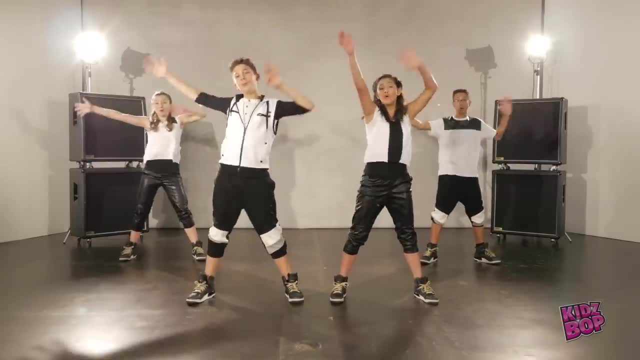 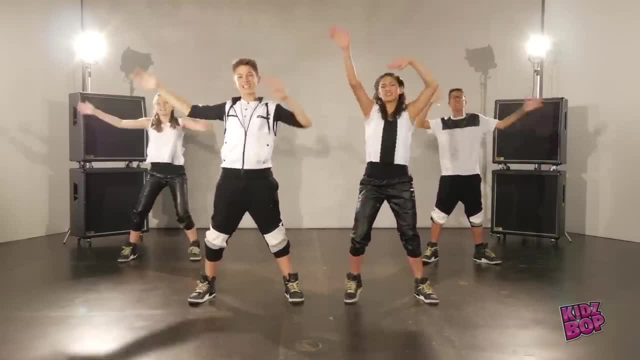 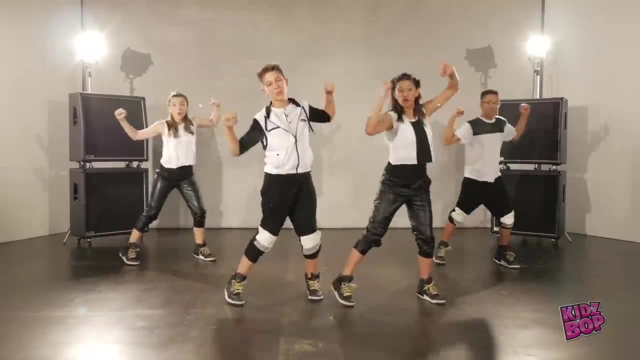 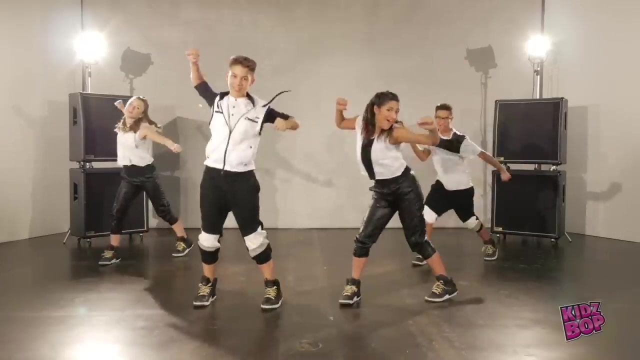 Let's get loud, loud, loud, loud, loud. Make some noise. Woo Scream out loud, twist, twist and shout. Do whatever you want to, And if you're stuck in the middle, Move it just a little And I bet you won't feel so blue. 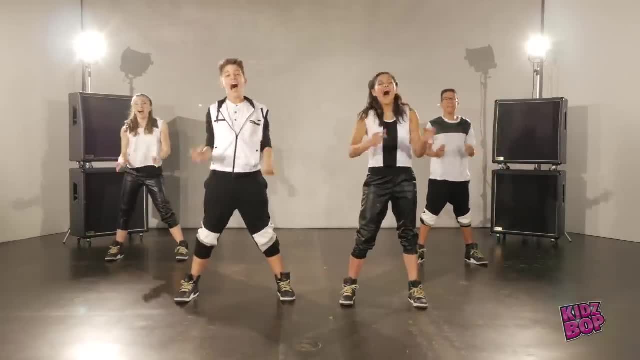 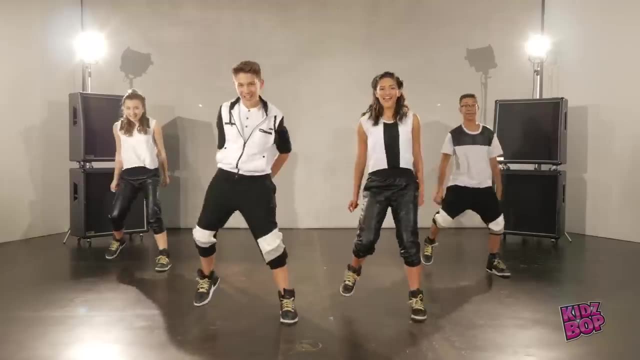 No, Soundly, do you feel? the speakers bumpin'. I ain't stoppin' till the Hall room's jumpin'. It's okay to get crazy now and then. Hey, Five, four, three, two, one. I feel like turnin' it up, breakin' it down. 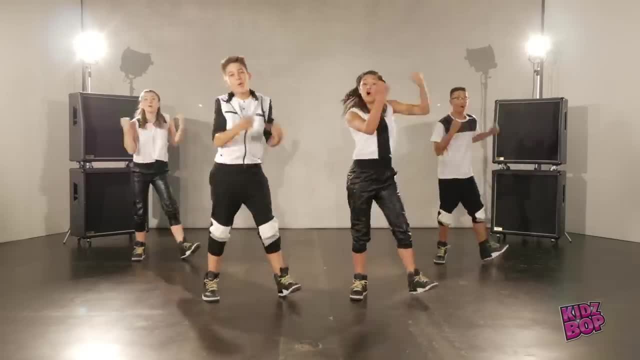 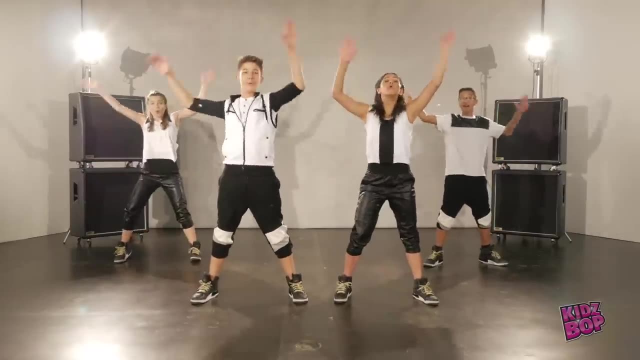 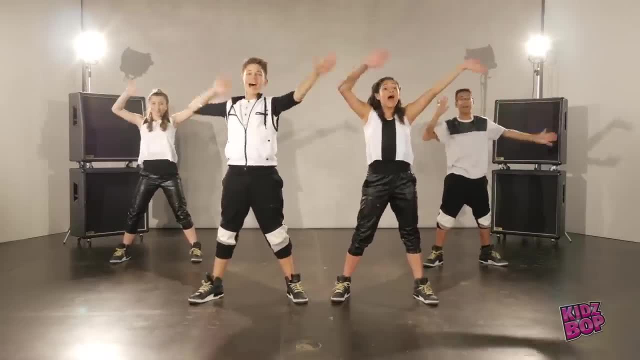 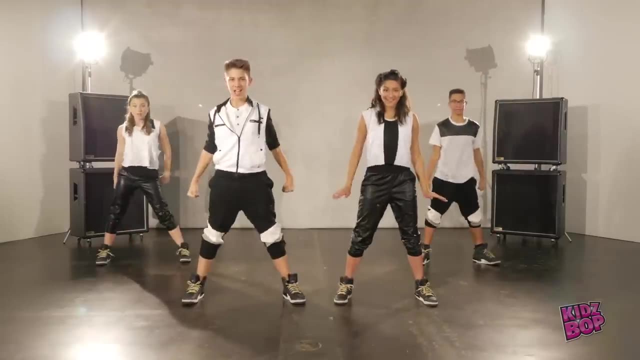 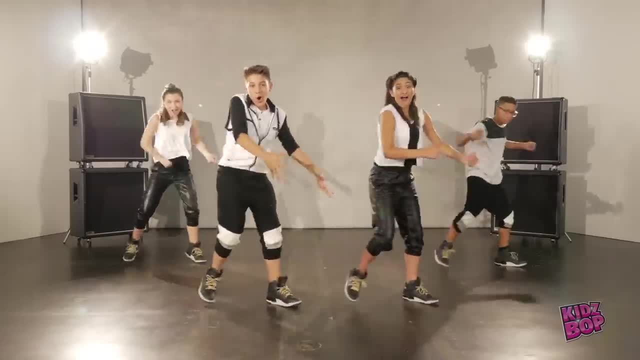 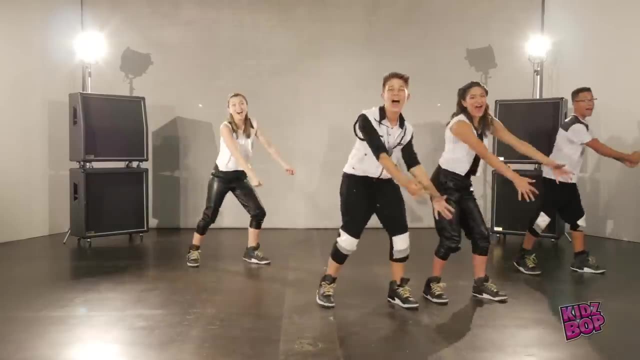 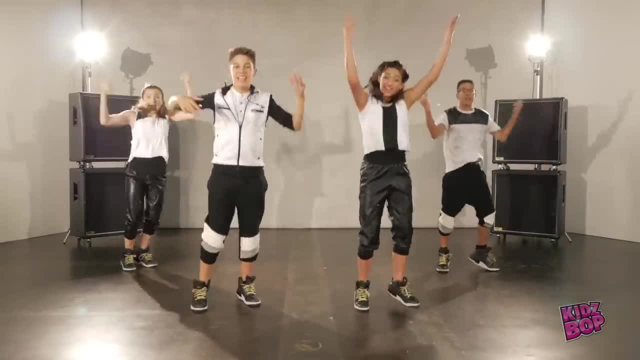 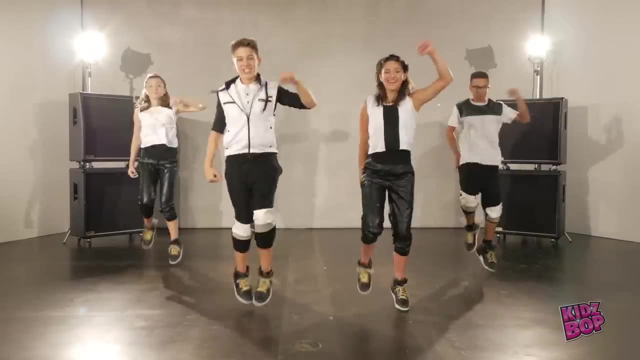 Get loud, loud, loud, loud, loud. Get loud, loud, loud, loud, loud. Get loud, loud, loud, loud, loud. Oh Yeah, loud, loud, loud, loud, loud. I wanna get loud Five, four, three, two, one. 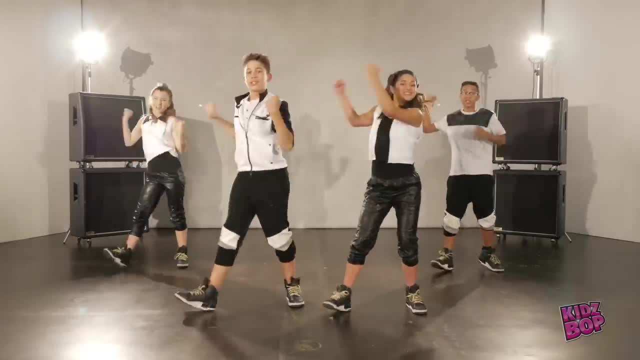 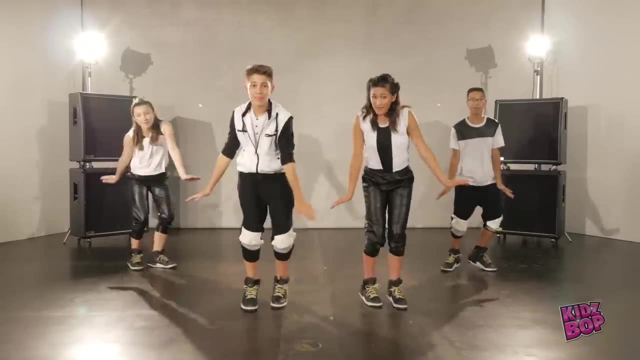 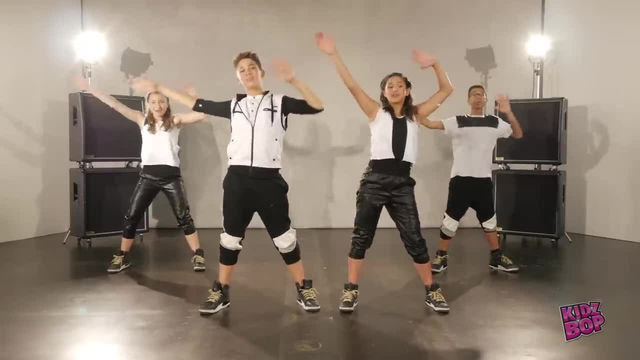 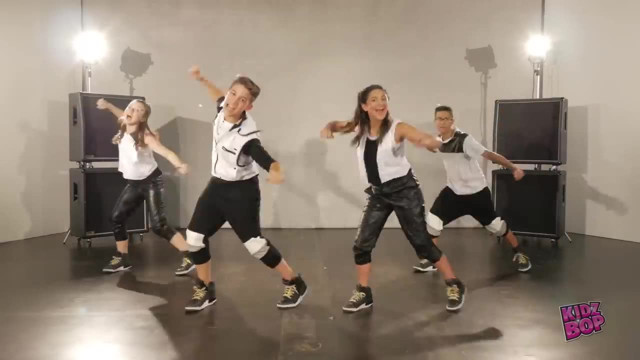 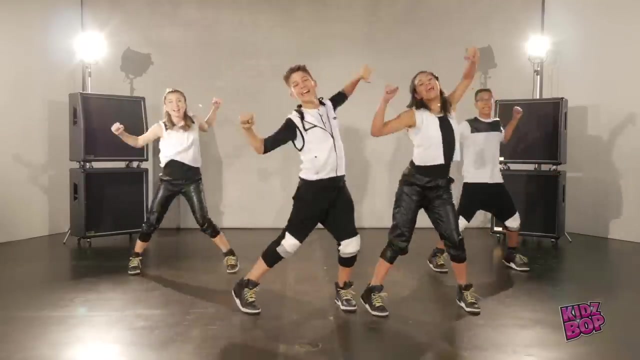 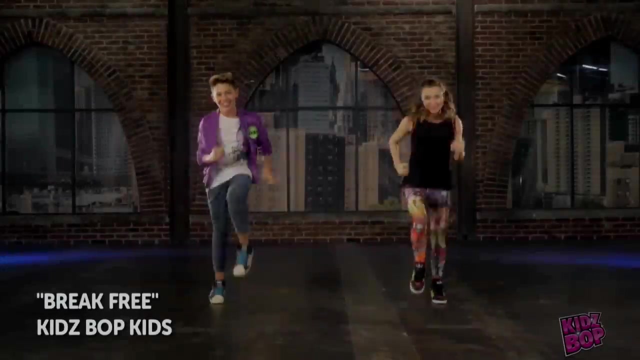 Ooh-ooh-ooh-ooh-ooh-ooh-ooh-ooh-ooh-ooh-ooh-ooh-ooh-ooh-ooh-ooh-ooh-ooh-ooh-ooh-ooh-ooh-ooh-ooh-ooh-ooh-ooh-ooh-ooh-ooh-ooh-ooh-ooh-ooh-ooh-ooh-ooh-ooh-ooh-ooh-ooh-ooh-ooh-ooh-ooh-ooh-ooh-ooh-ooh-ooh-ooh-ooh-ooh-ooh-ooh-ooh-ooh-ooh-ooh-ooh-ooh-ooh-ooh-ooh-ooh-ooh-ooh-ooh-ooh-ooh-ooh-ooh-ooh-ooh-ooh-ooh-ooh-ooh-ooh-ooh-ooh-ooh-ooh-ooh-ooh-ooh-ooh-ooh-ooh-ooh-ooh-ooh-ooh-ooh-ooh-ooh-ooh-ooh-ooh-ooh-ooh-ooh-ooh-ooh-ooh-ooh-ooh-ooh-ooh-ooh-ooh-ooh. 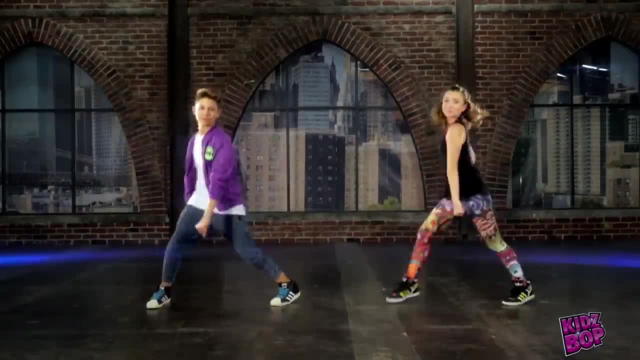 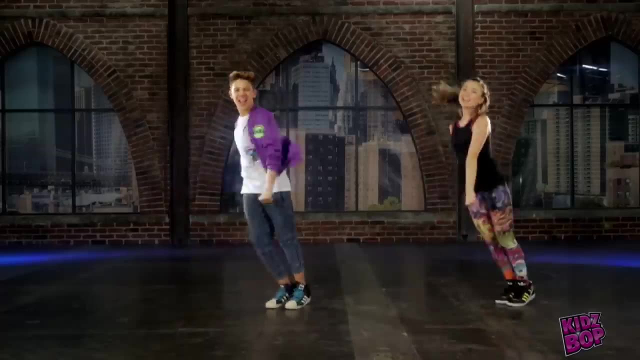 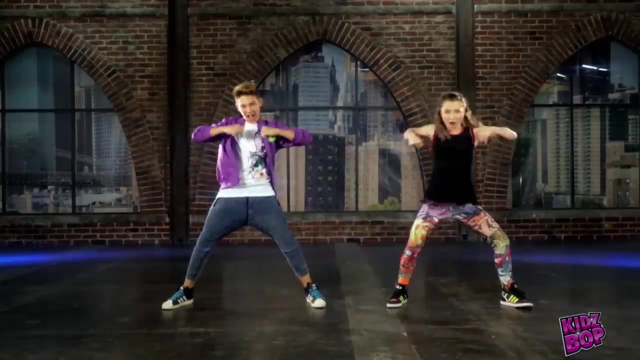 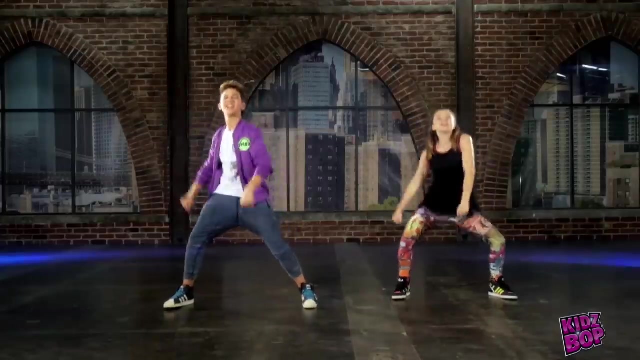 If you want it, Take it. I should've said it before. Try to hide it, Fake it. I can't pretend anymore. I only wanna come alive, Never by the hands of a broken heart. Don't wanna hear you lie, or not, Now that I've become who I really am. 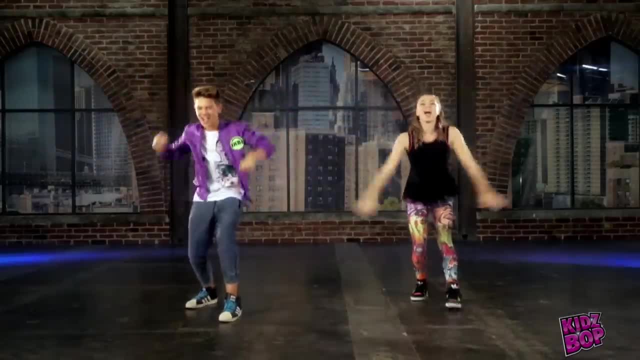 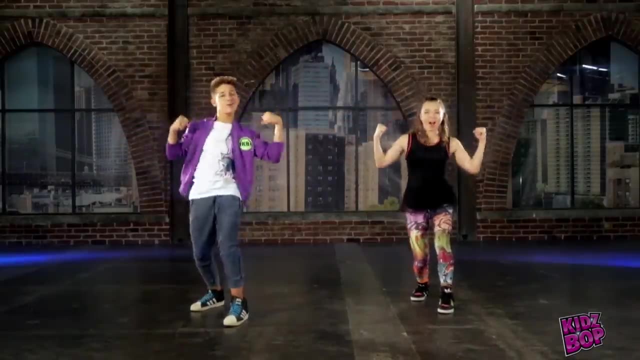 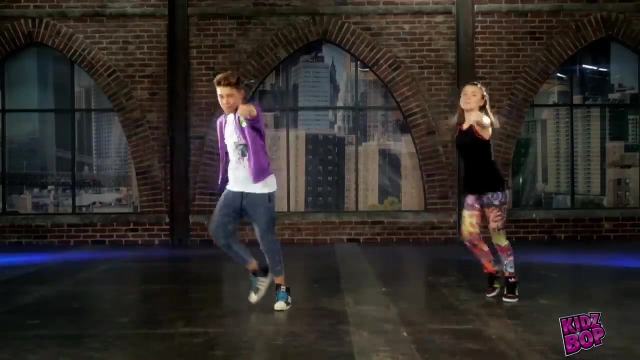 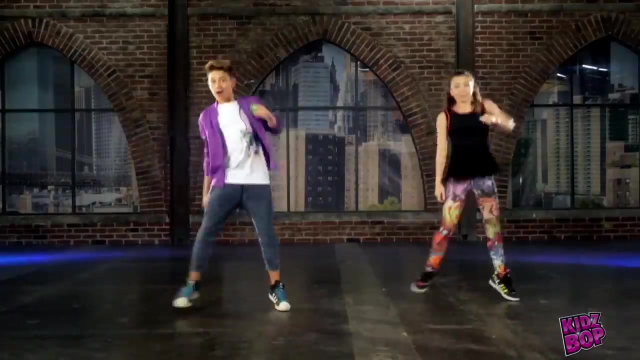 This is The part when I say: I don't wanna. I'm stronger than I've been before. This is The part when I break free Cause I can't resist it no more. This is The part when I say: I don't wanna. I'm stronger than I've been before. This is The part when I break free. 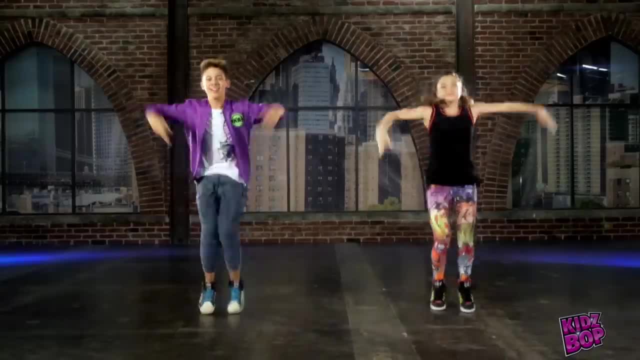 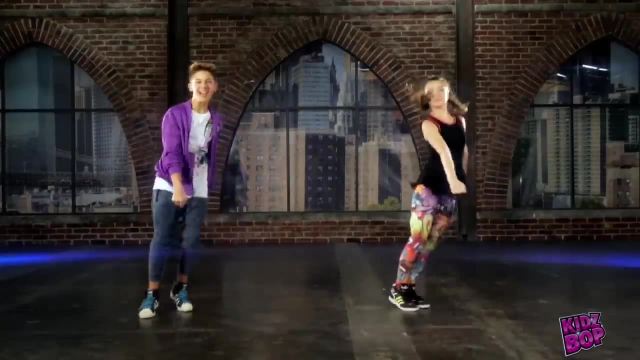 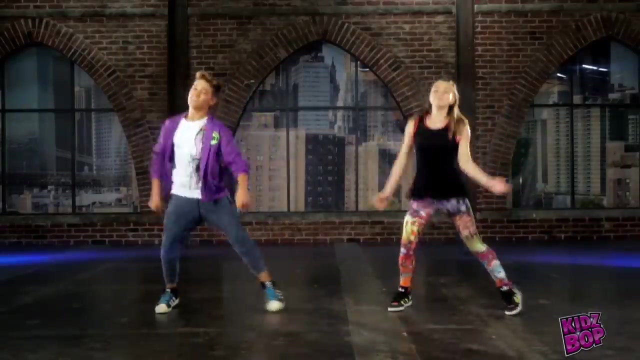 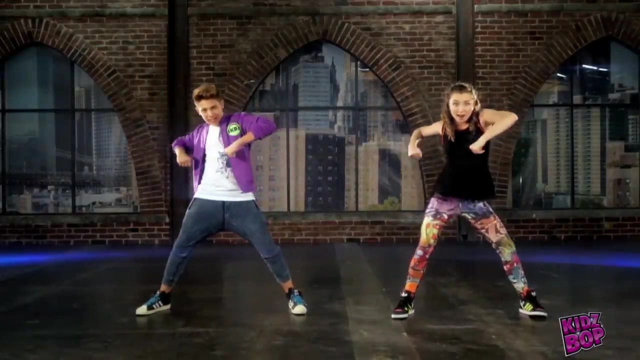 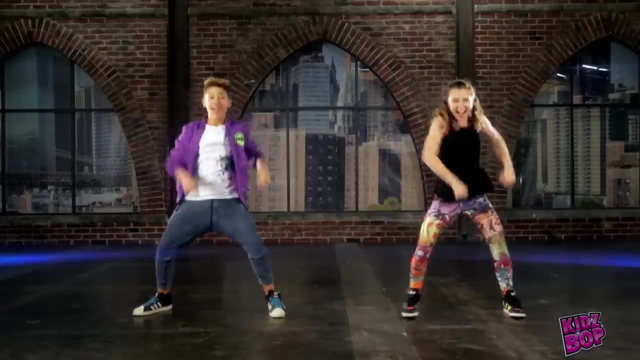 You were better Freer. I was under your spell Like a hydrant. Feel my air, babe, On the highway of failure, I only wanna come alive, Never by the hands of a broken heart. Don't wanna hear you lie or not. Now that I've become who I really am, 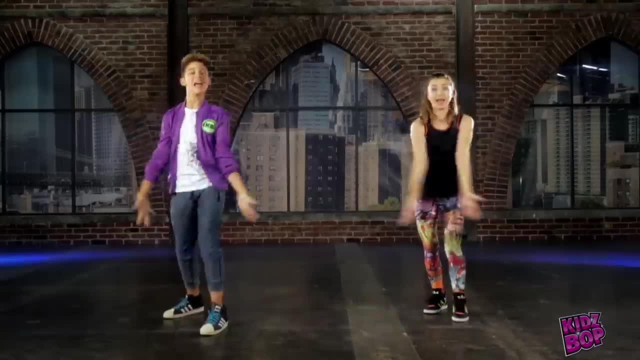 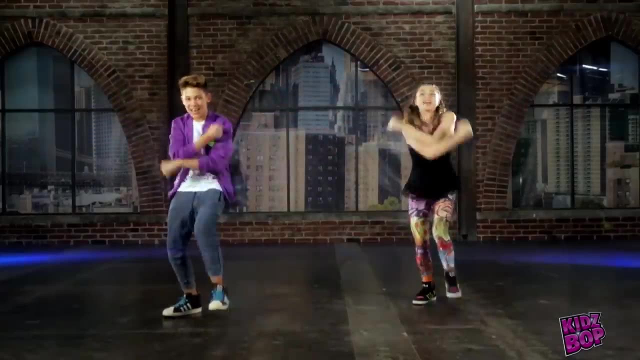 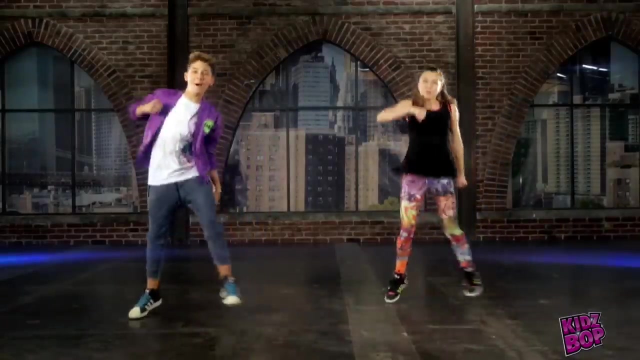 This is The part when I say: I don't wanna. I'm stronger than I've been before. This is The part when I break free Cause I can't resist it no more. This is The part when I say: I don't wanna. I'm stronger than I've been before. 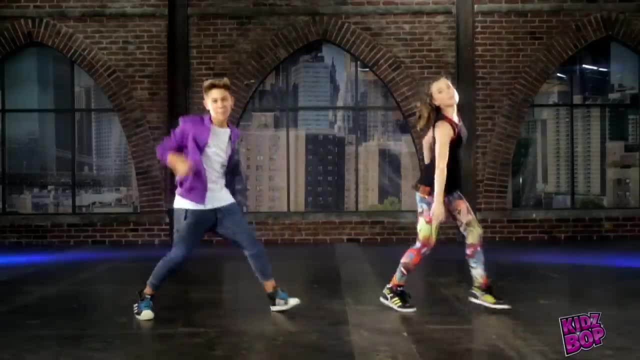 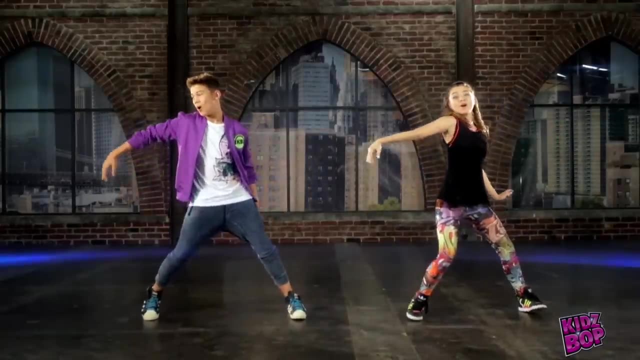 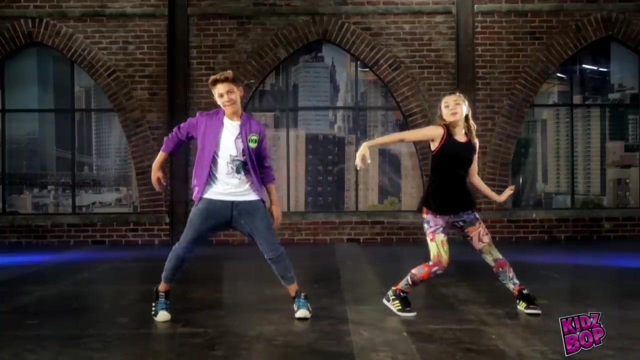 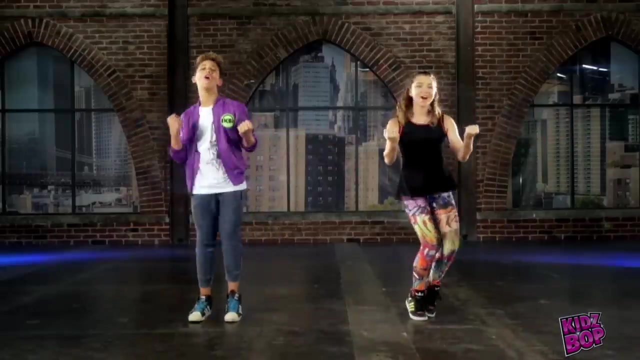 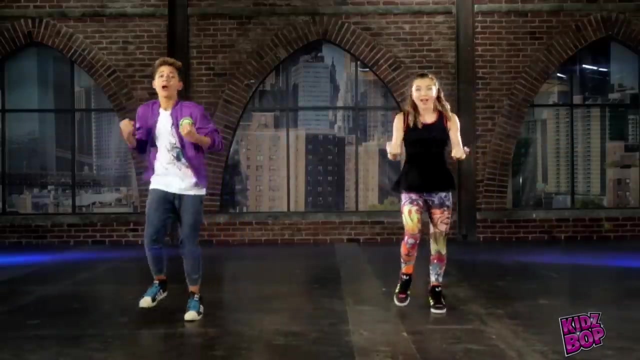 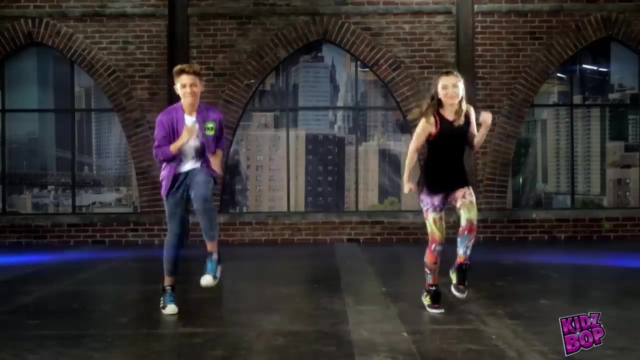 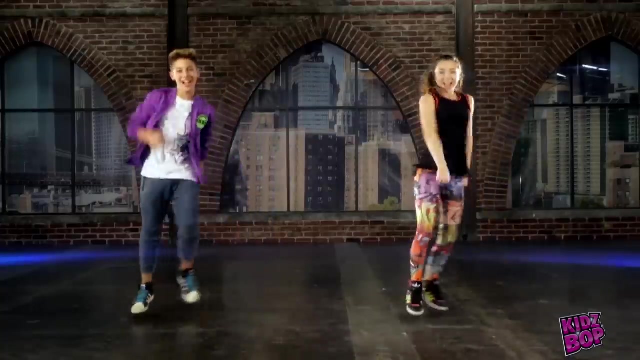 This is The part when I break free Cause I can't resist it. no more. No more baby. Mind over body. I came alive. It was futile, it was fever. In my dreams, it felt so right, But I woke up every time: Oh baby. This is The part when I say: I don't wanna. I'm stronger than I've been before. 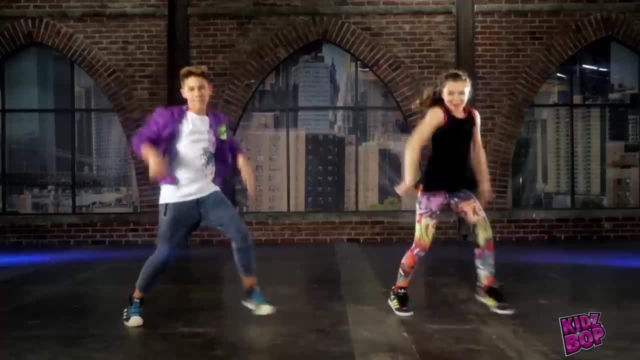 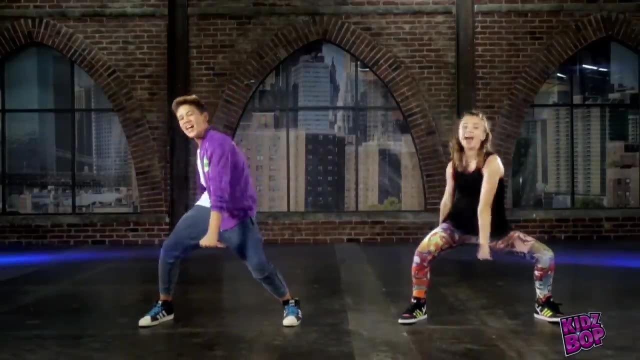 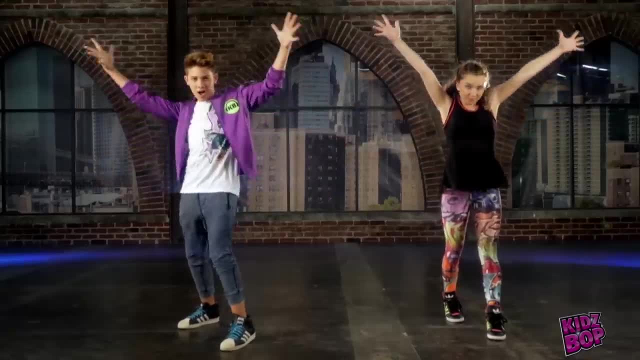 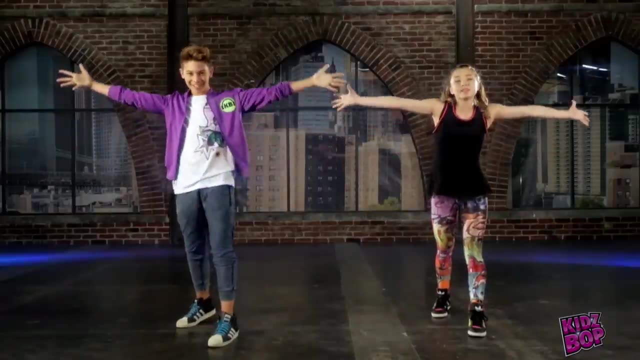 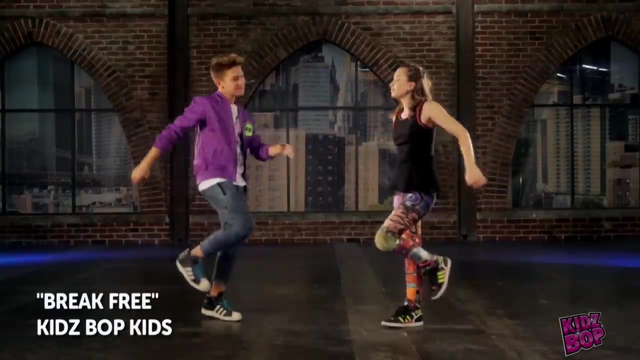 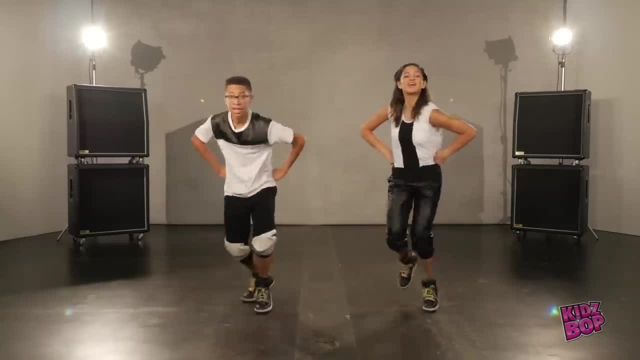 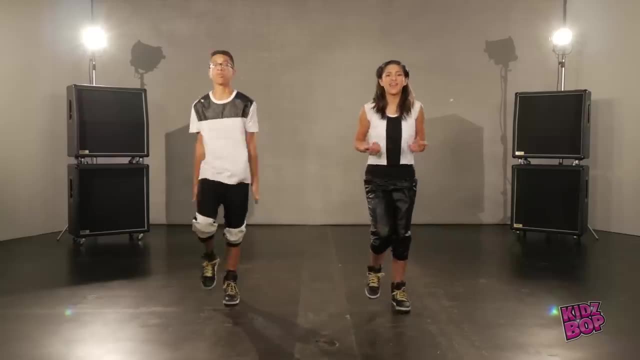 I'll be your light, your match, your burning sun. I'll be the bright and black that's making you run And we'll feel alright. and we'll feel alright Cause we'll work it out. yeah, we'll work it out. I'll be doing this if you have a doubt. 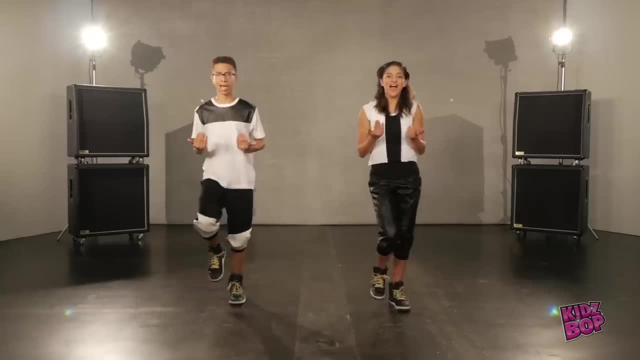 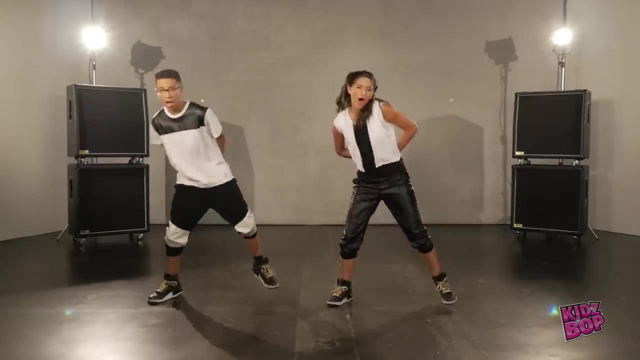 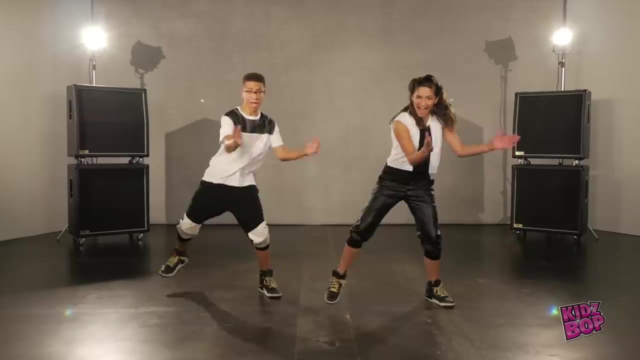 Till the love runs out. till the love runs out, I'll be your ghost, your game, your stadium. I'll be your fifth, two thousand clapping like one, And I'll feel alright. and I'll feel alright Cause I've worked it out. yeah, I've worked it out. 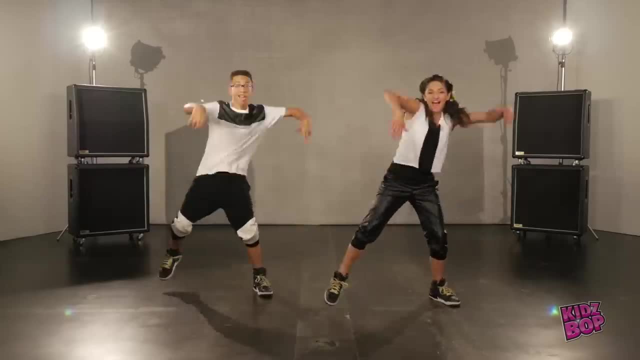 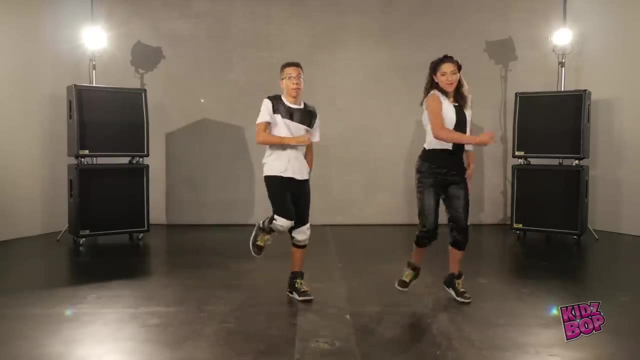 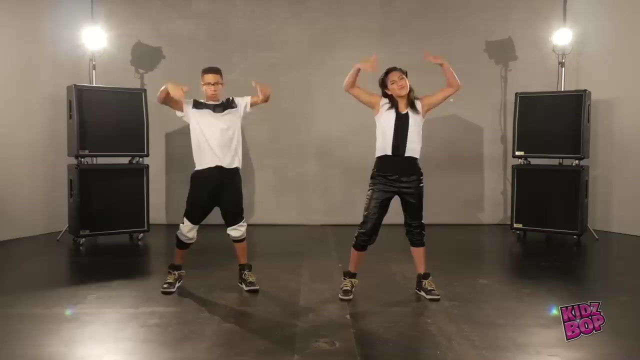 I'll be doing this, if you have a doubt, Till the love runs out. till the love runs out, I got my mind made up and I can't let go. I'm going everywhere. Second to this is my soul. I'll be running. I'll be running. 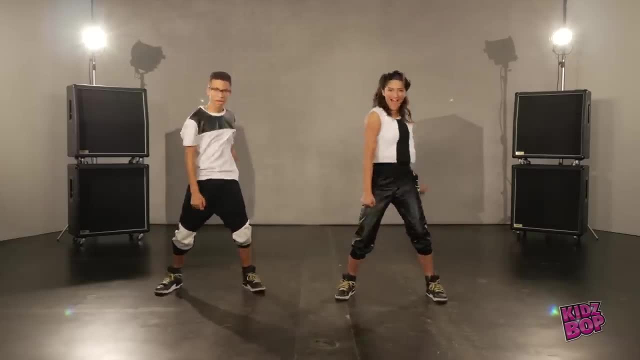 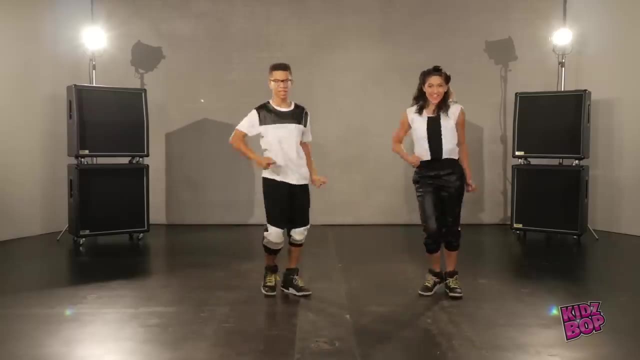 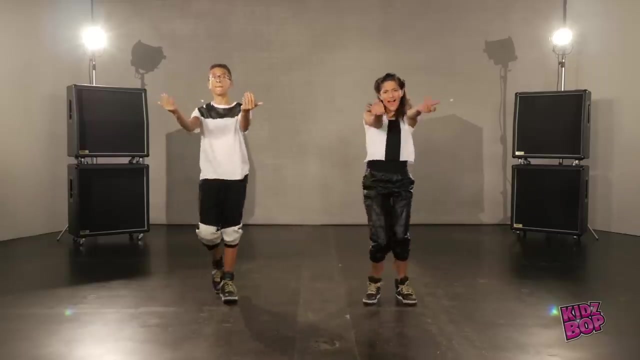 Till the love runs out. till the love runs out, And we'll start a fire and we'll shut it down Till the love runs out. till the love runs out. There's a maniac out in front of me, Got an angel on my shoulder, and if he wants to meet, 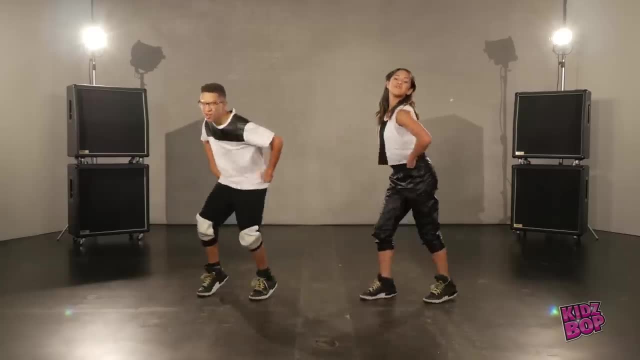 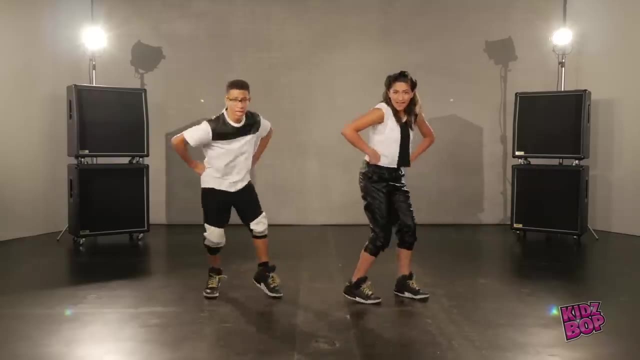 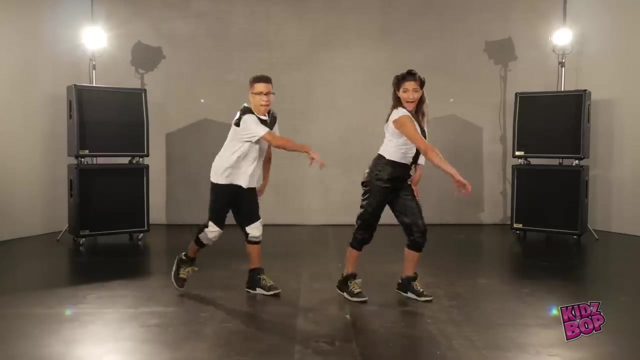 But mama raised me, good, mama raised me right. Mama said: do what you want, say prayers tonight- And I'm saying man, cause I'm so devout- Till the love runs out. till the love runs out, I got my mind made up and I can't let go. 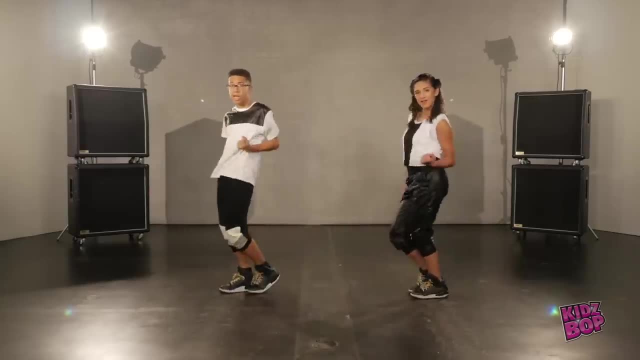 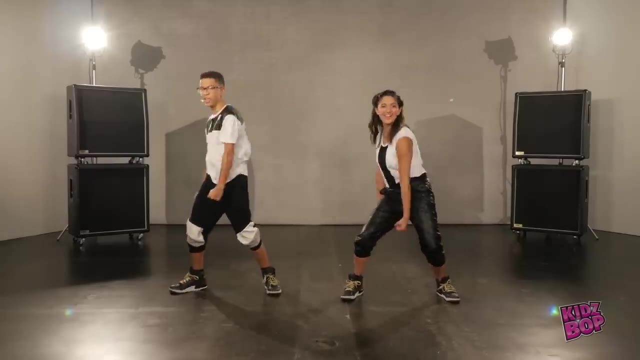 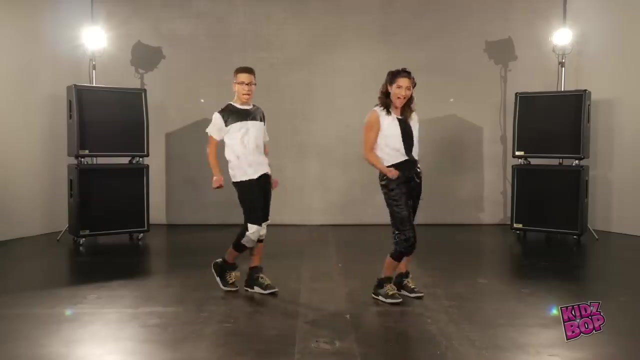 I'm going every second till it sees my soul. I'll be running. I'll be running Till the love runs out, till the love runs out, And we'll start a fire And we'll shut it down Till the love runs out, till the love runs out. 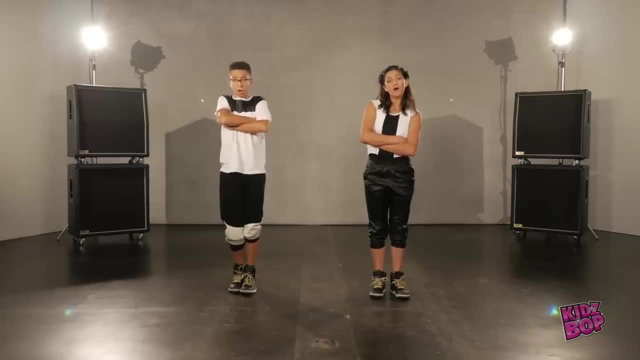 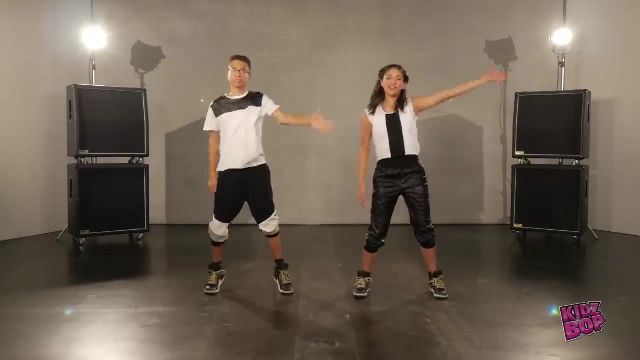 Oh, we all want the same thing. Oh, we all run for something. Run for God, for faith, for love, for hate, For God, for us, for diamonds. I'll be your light, your match, your burning sun. I'll be the bright and black that's making you run. 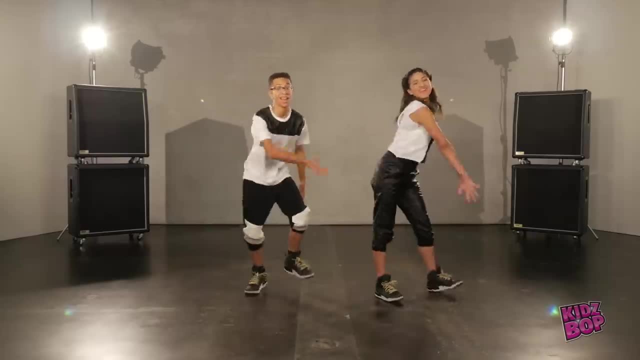 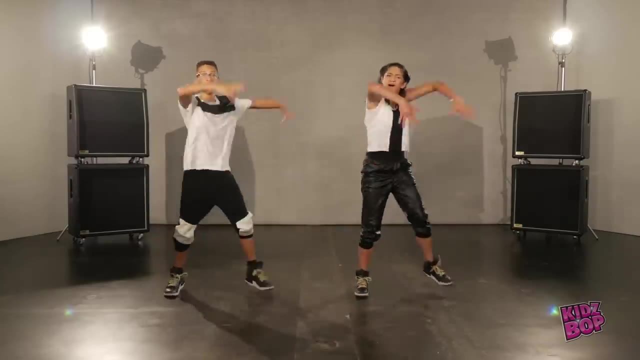 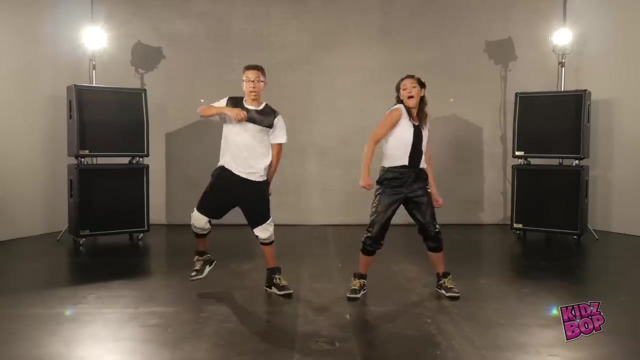 I got my mind made up and I can't let go. I'm going every second till it sees my soul. I'll be running, I'll be running Till the love runs out, till the love runs out, And we'll start a fire and we'll shut it down. 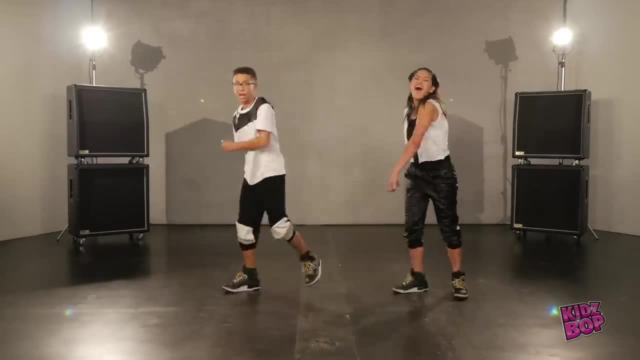 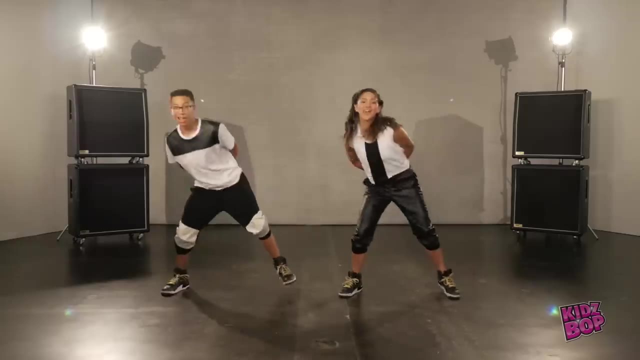 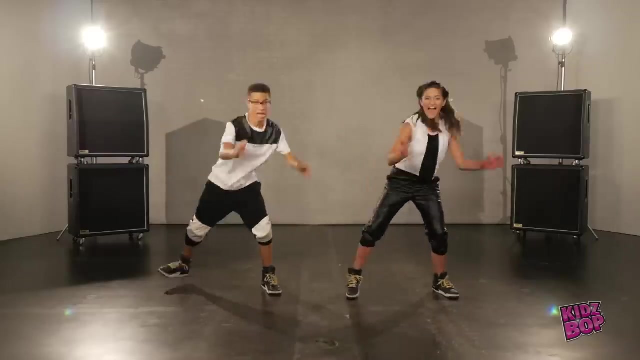 Till the love runs out. till the love runs out, I'll be your light, your match, your burning sun. I'll be the bright and black that's making you run And we'll speak for all. and we'll speak for all And cause. we'll work it out. yeah, we'll work it out. 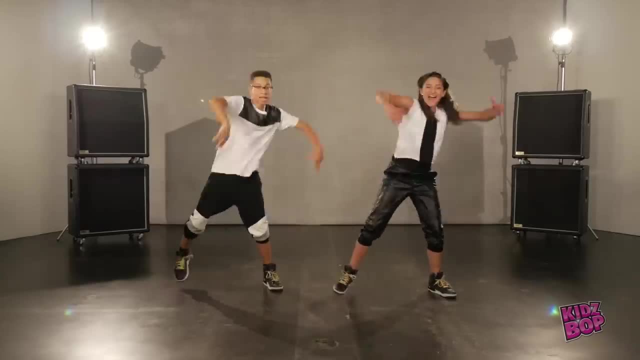 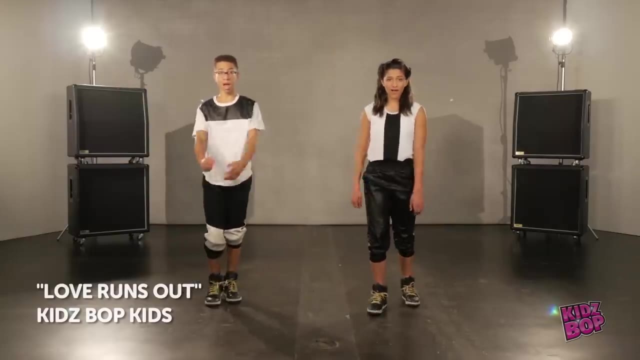 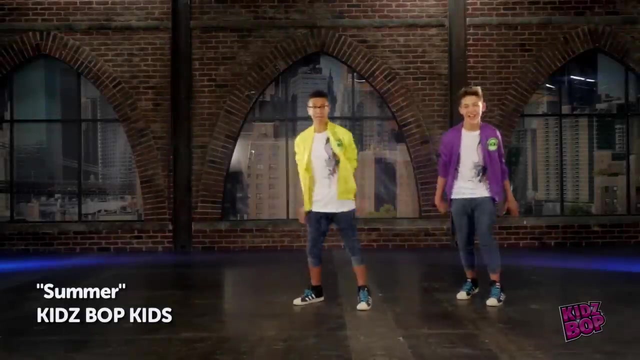 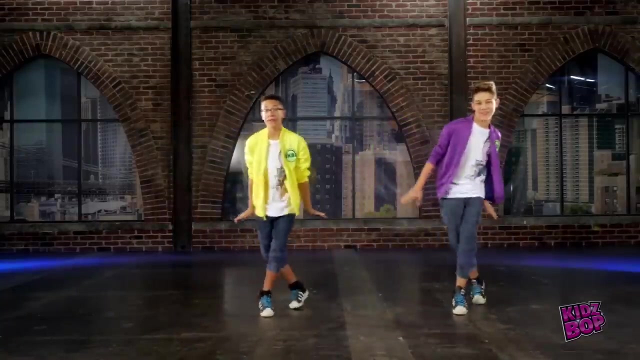 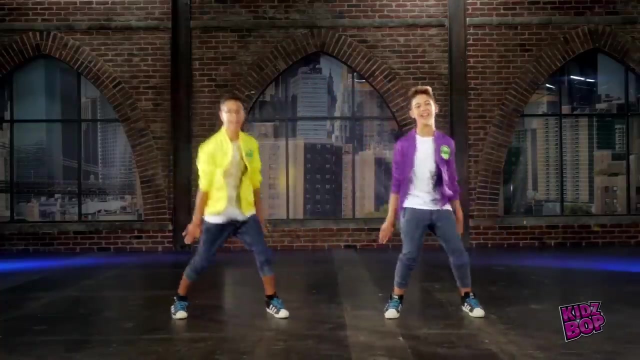 And we'll start a fire and we'll shut it down Till the love runs out. till the love runs out, Till the love runs out. When I met you in the summer, Till my heart beat sound, We fell in love. As the leaves turned brown, We could be together, baby. 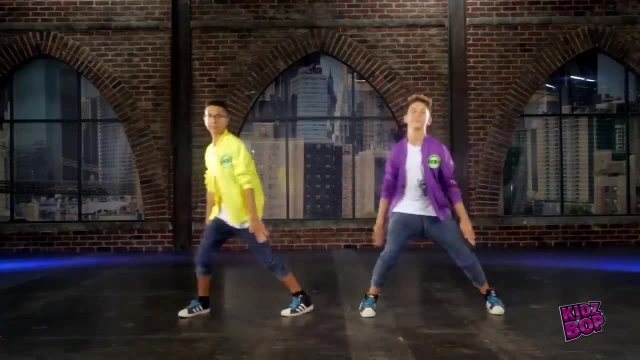 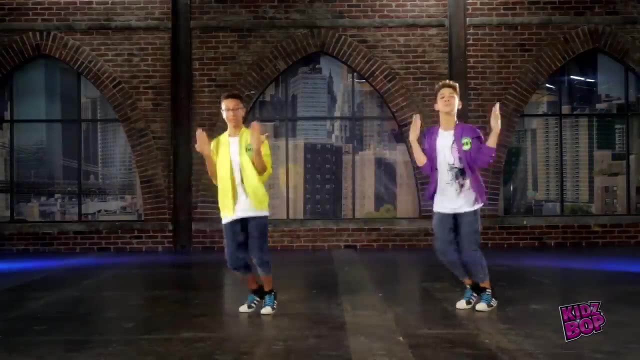 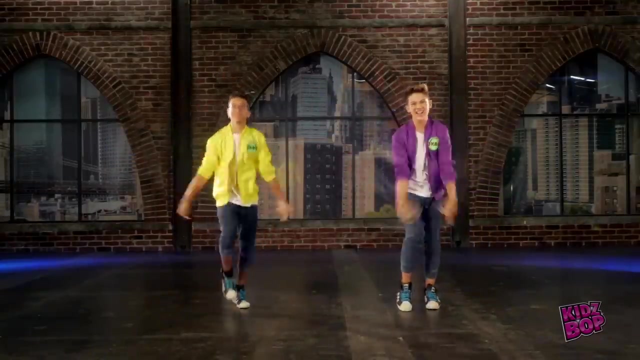 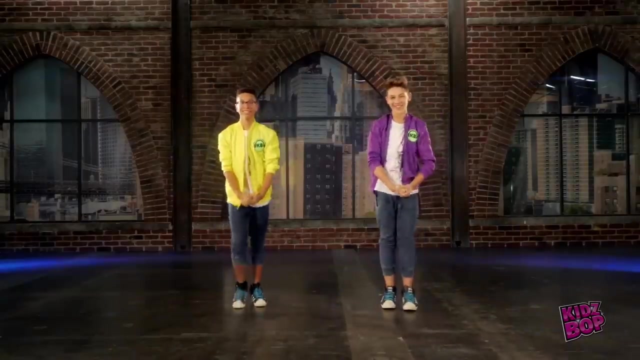 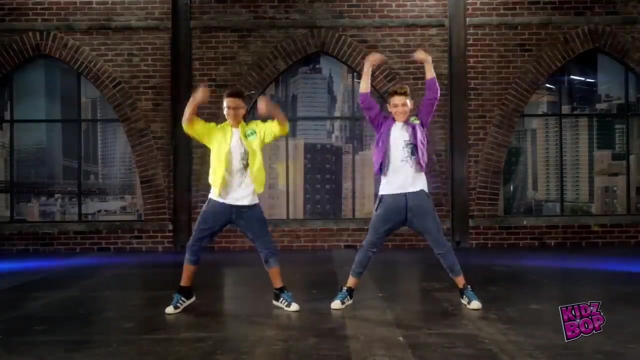 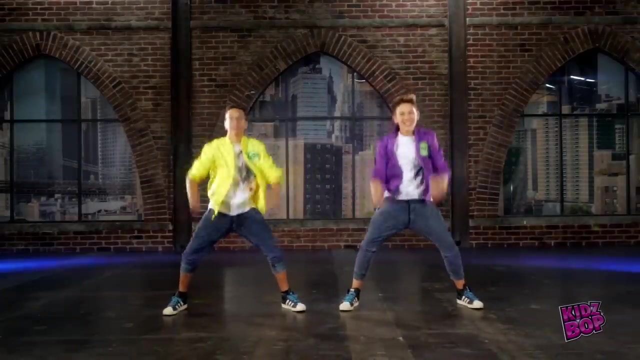 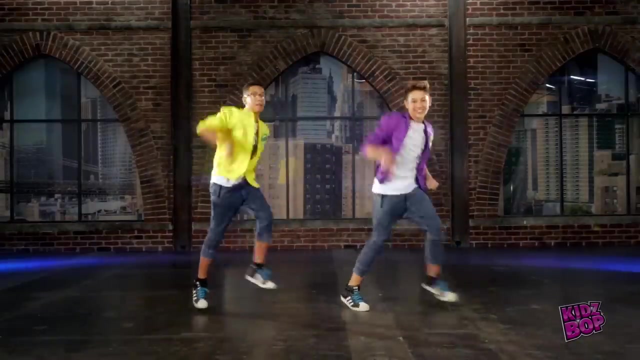 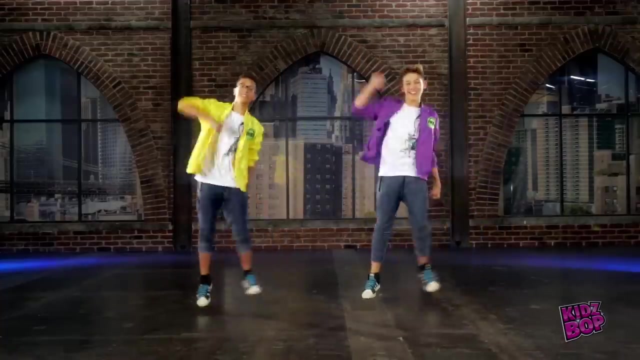 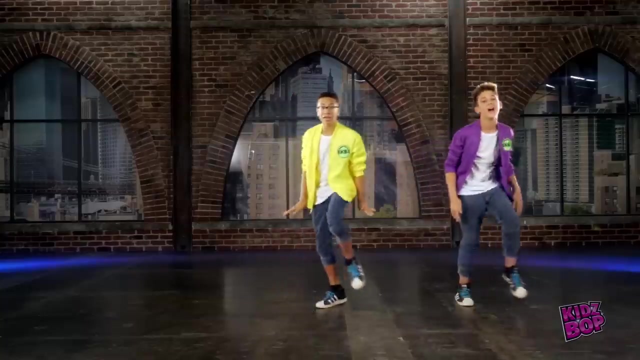 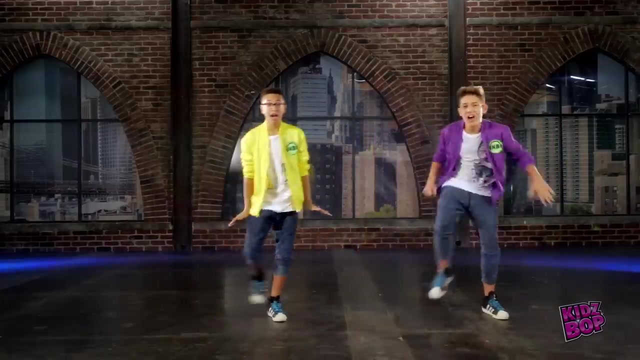 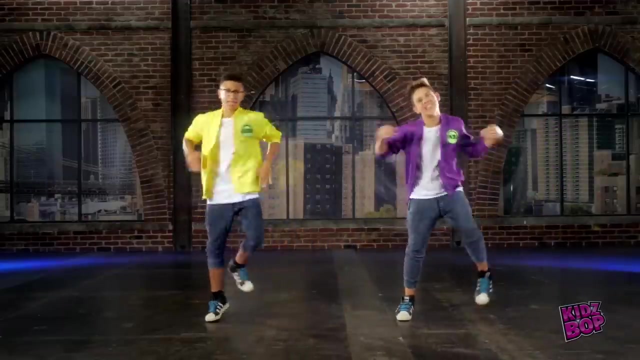 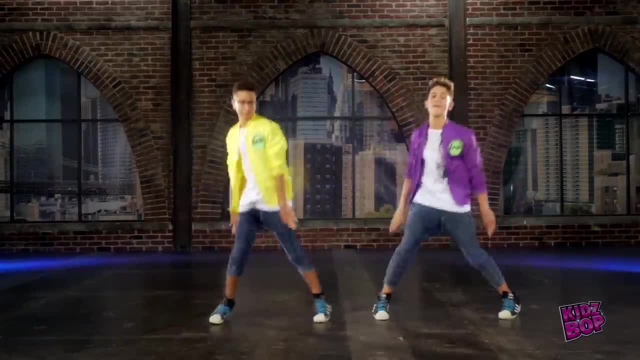 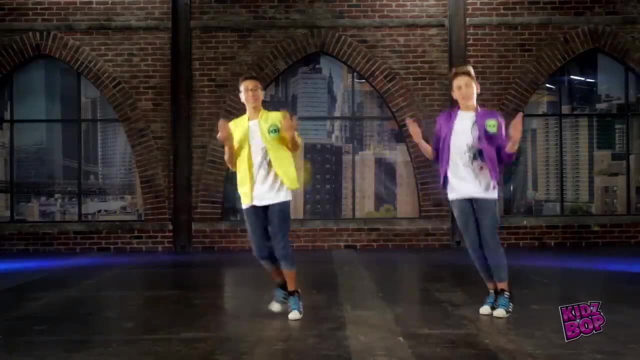 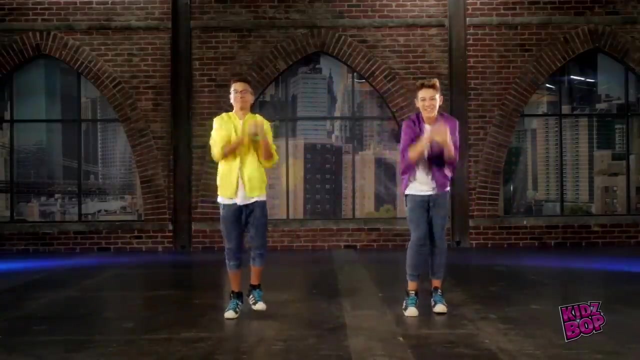 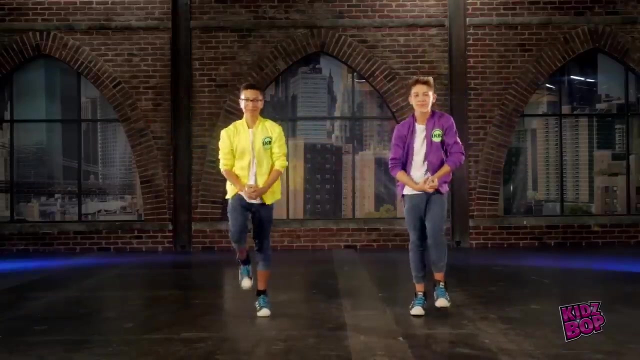 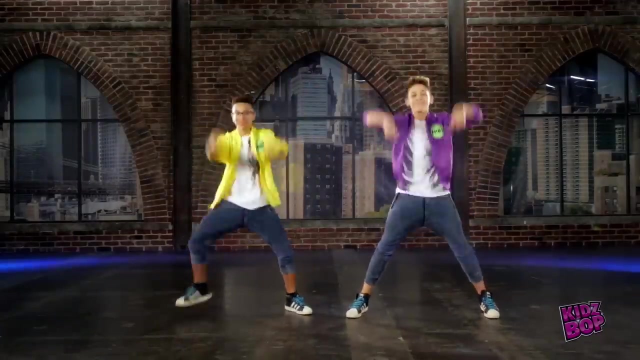 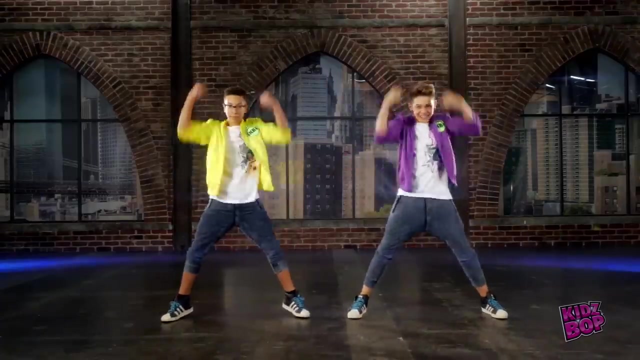 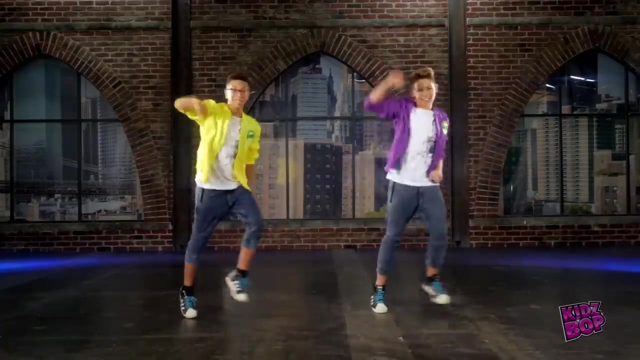 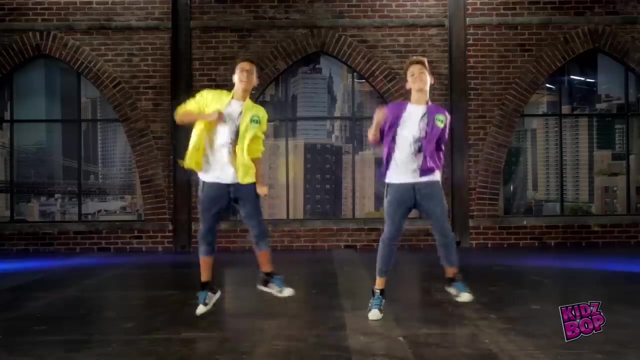 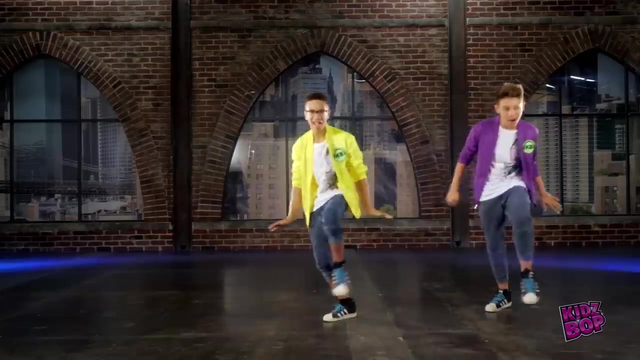 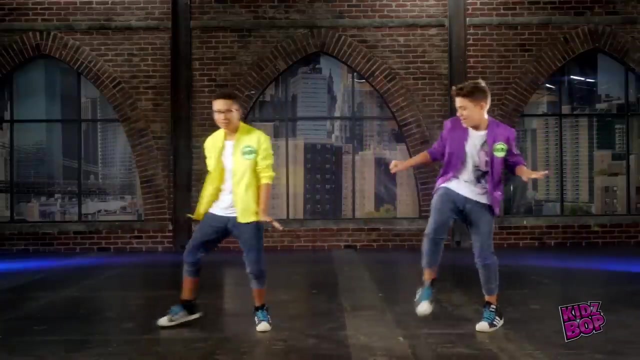 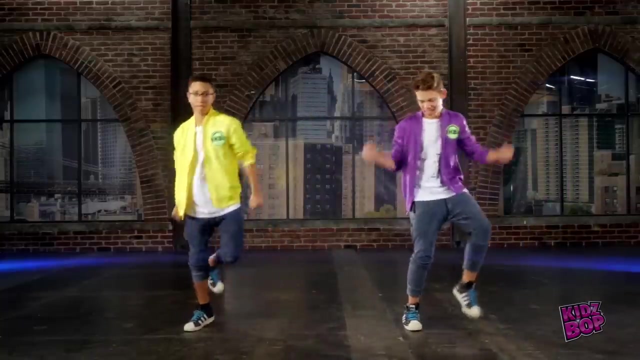 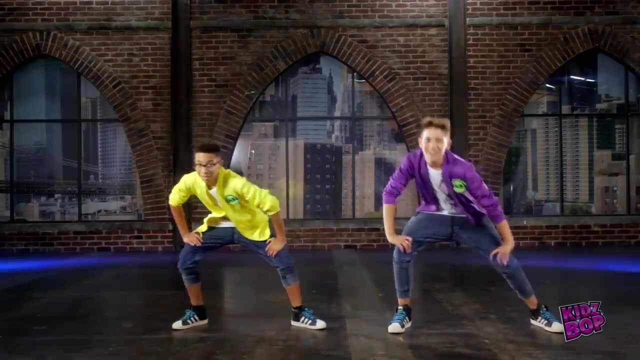 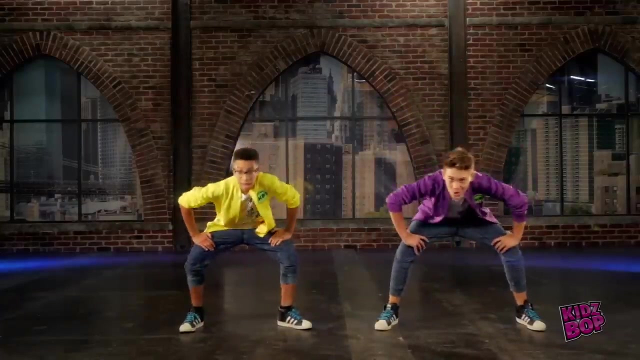 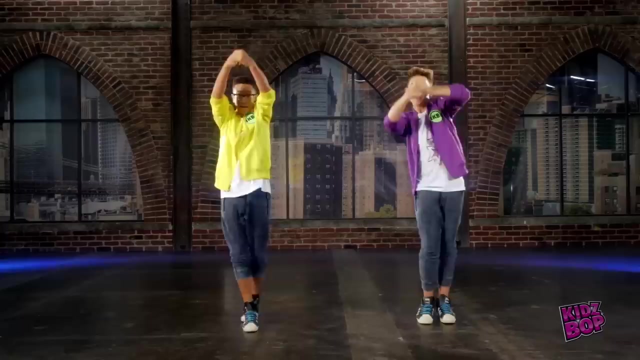 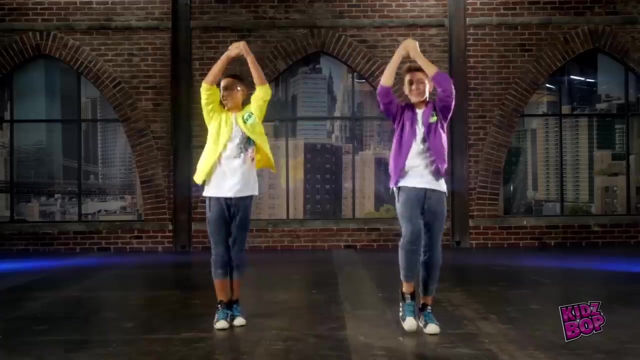 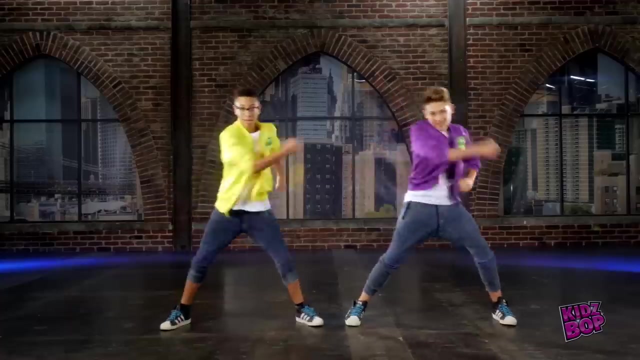 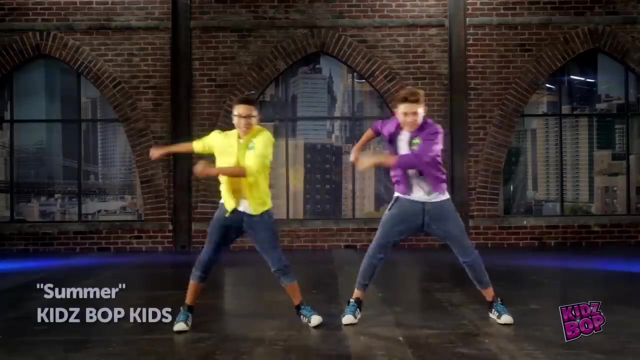 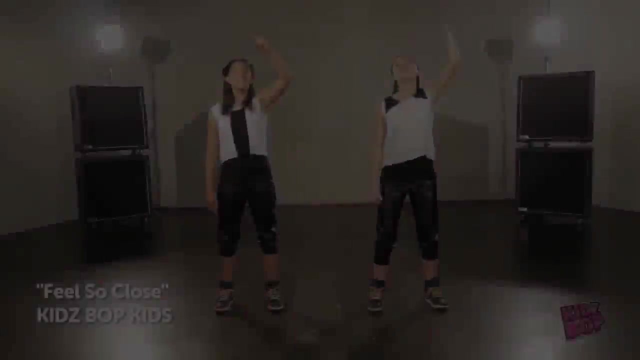 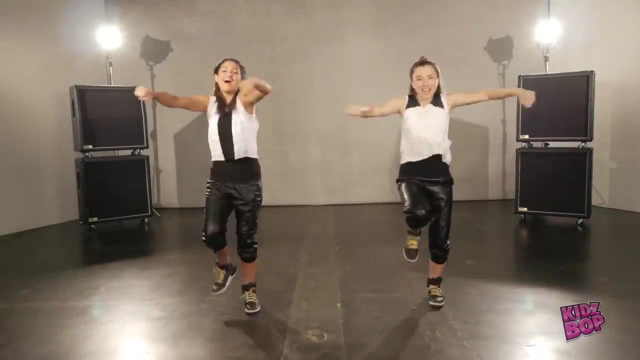 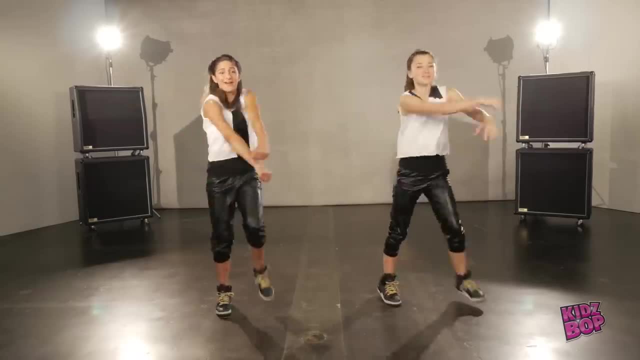 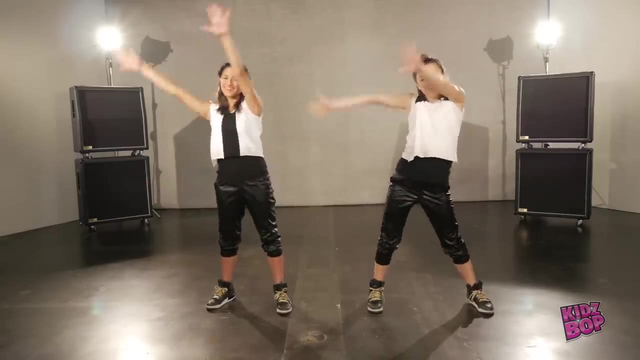 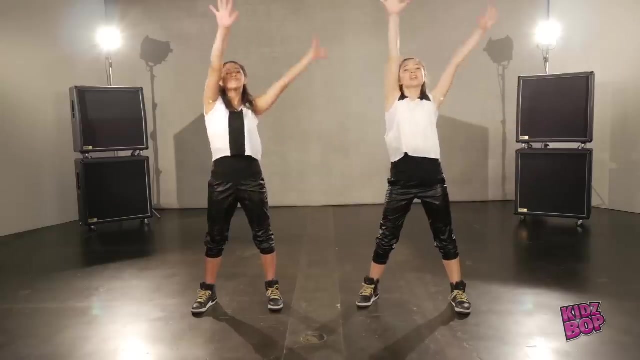 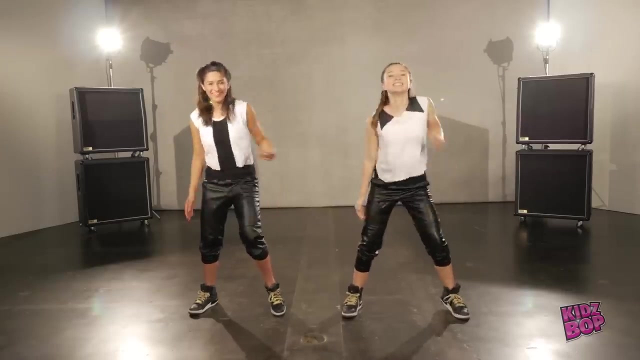 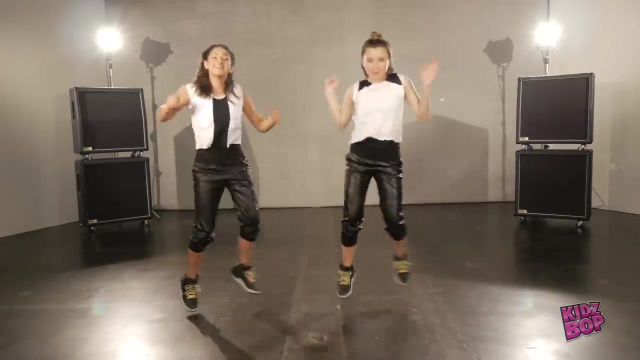 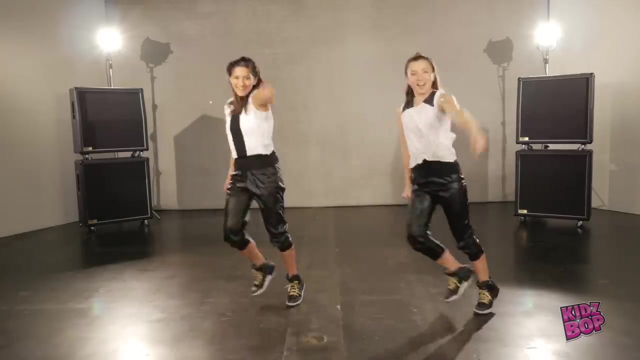 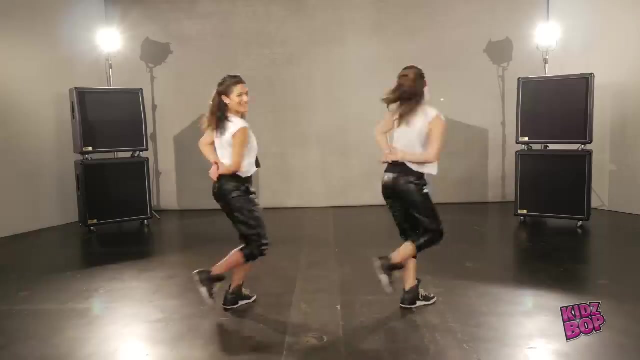 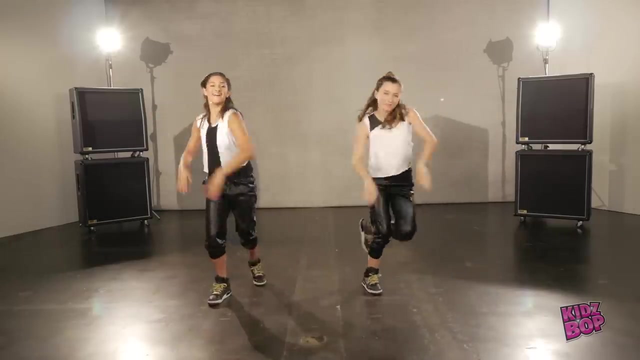 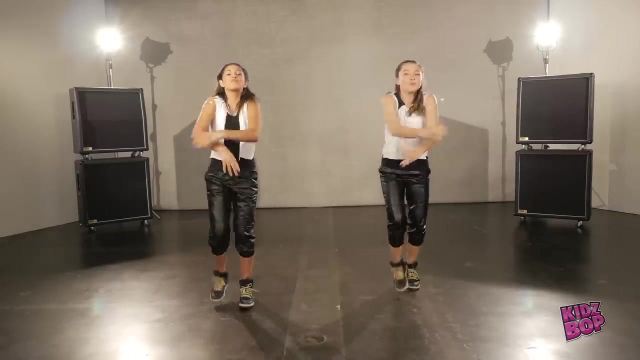 Like a big deal. Your love pours down on me, Surround me like a waterfall And there's no stopping us. right now, I feel so close to you. I feel so close to you right now. I feel so close to you right now. It's a force field. I wear my heart upon my sleeve. 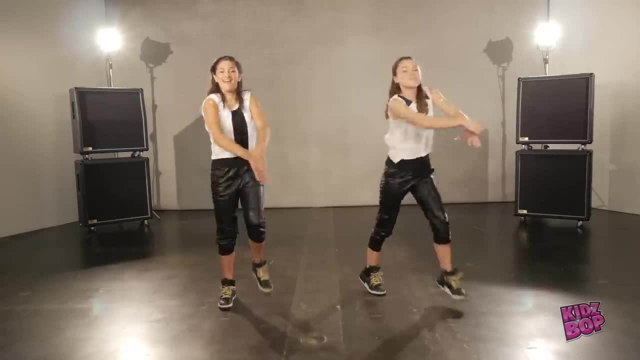 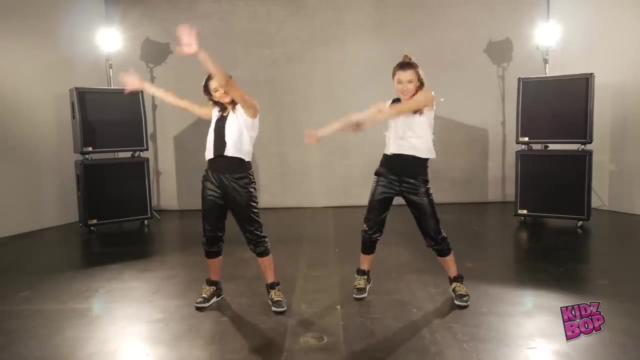 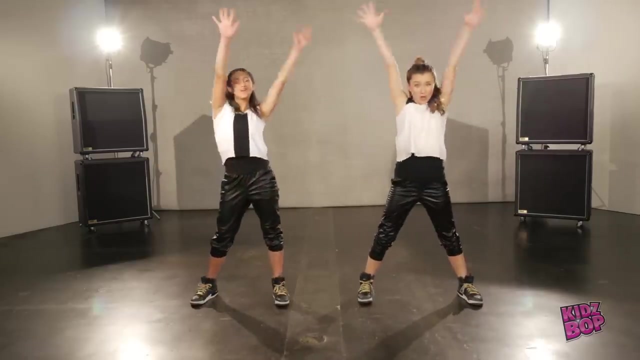 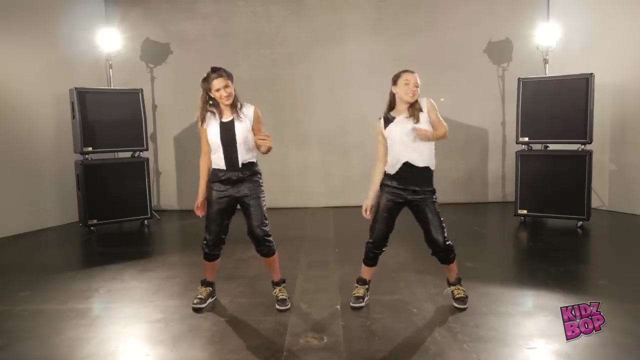 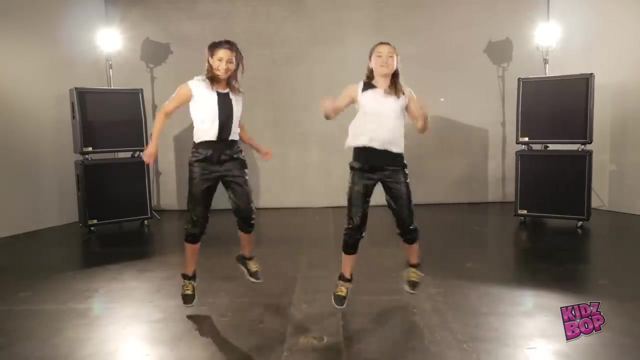 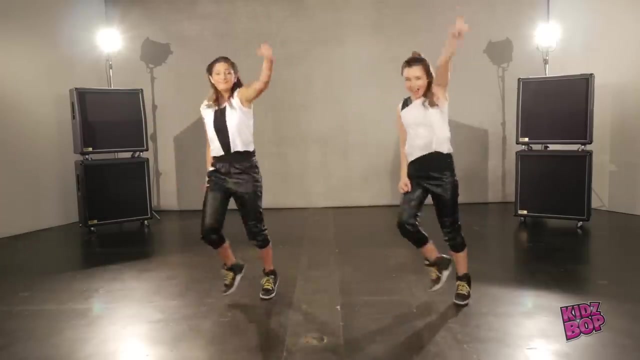 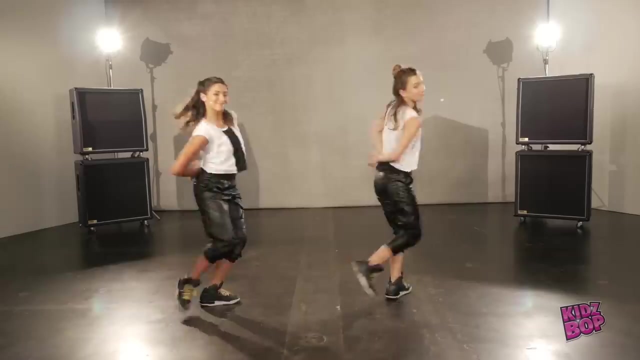 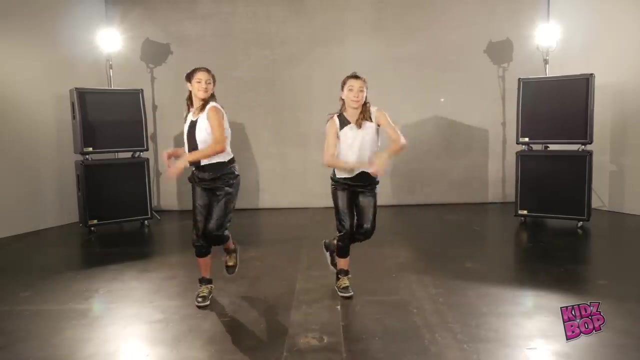